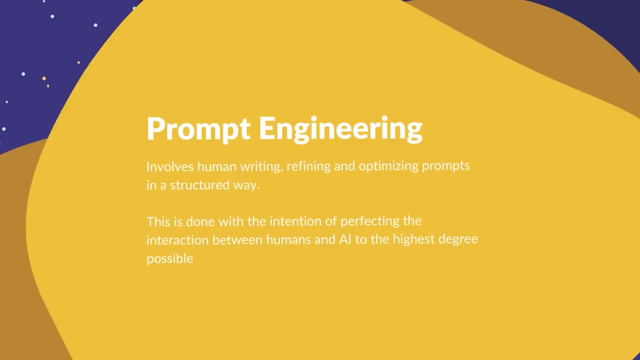 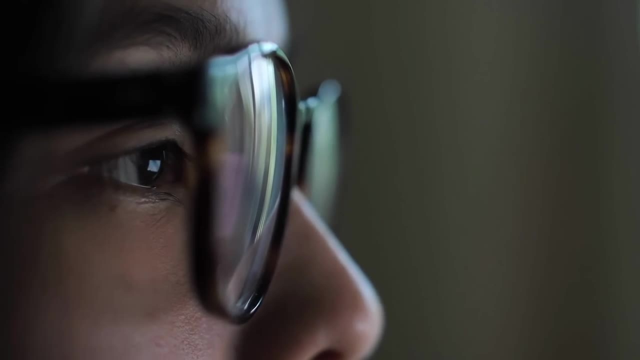 between humans and AI to the highest degree possible. Not only that, however. a prompt engineer is then also required to continuously monitor those prompts to ensure their effectiveness with time and effort. So let's get started. 1. What is a prompt? 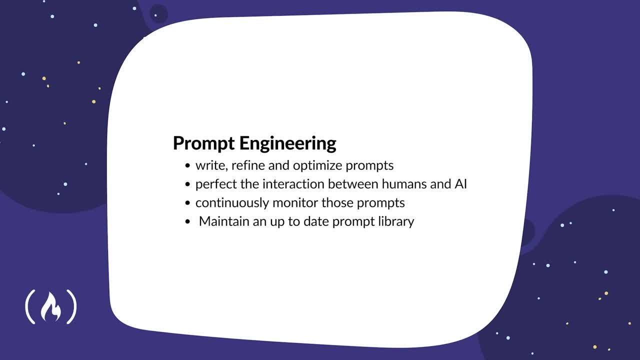 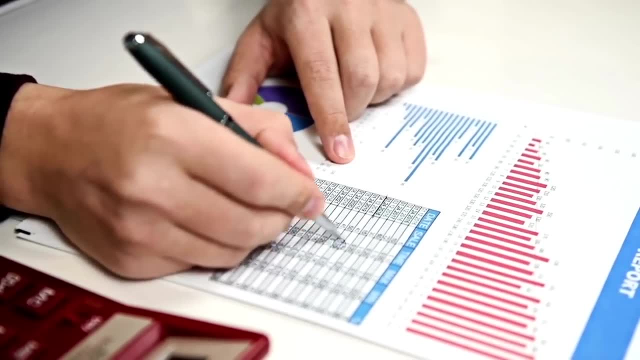 A prompt engineer works to monitor conversation time. as AI progresses, Maintaining an up-to-date prompt library will be a requirement that's placed onto the prompt engineer, as well as reporting on findings and, in general, being a thought leader in this space. But why do we need it and how did it come about from AI? 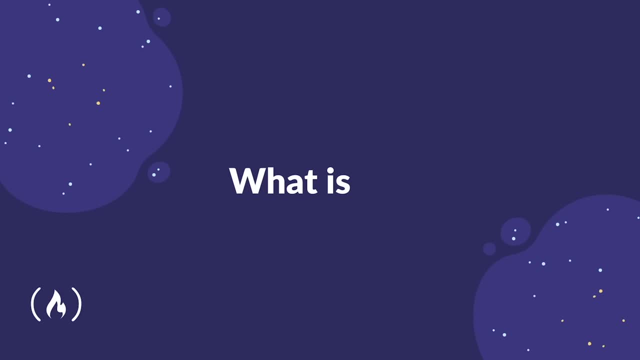 Before moving on, let's actually make sure we're on the same page about what exactly AI is. Artificial intelligence is the simulation of human intelligence processors by machines. I say simulation as often as we are losing the ability to experience artificial intelligence, which does not do the same to AI. This is why we cannot change the process of curve and behavior, as you understand AI, by using the internet. 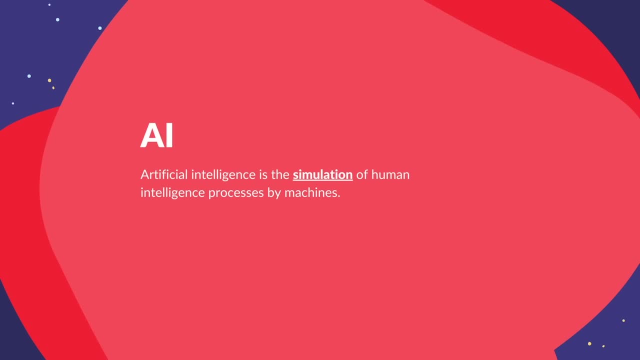 2. How do AI work? Artificial intelligence is the simulation of human intelligence processes by machines. I say simulation as artificial intelligence is not sentient, at least not yet anyways, meaning it cannot think for itself, as much as it may seem it does. 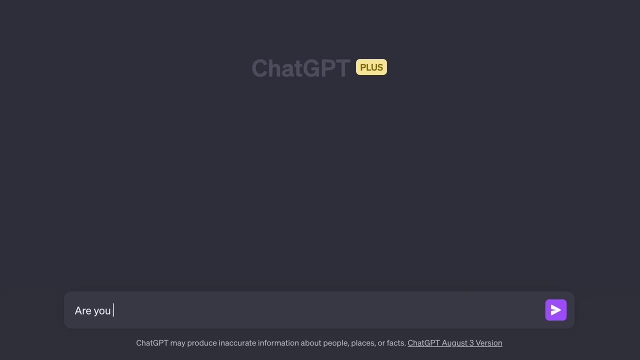 Often- and this is certainly the case with tools such as chat, GPT, for example- when we say AI, we are simply referring to a term called machine learning. Machine learning works by using large amounts of training data that is then analyzed for correlations and patterns. 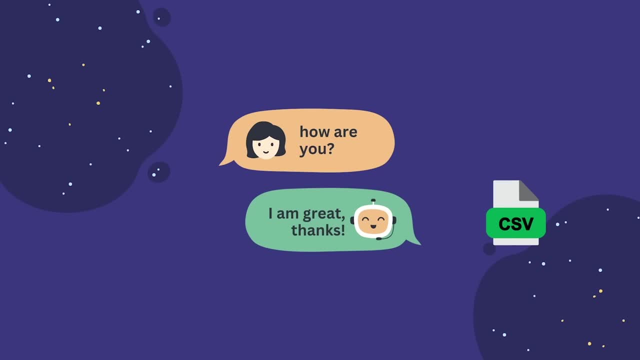 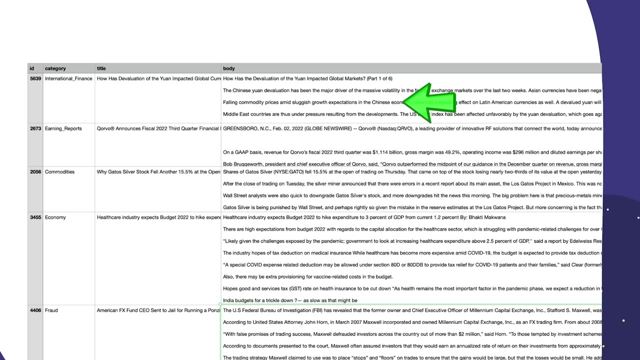 These patterns are then used to predict outcomes based on the training data provided. So, for example, here we are feeding data saying that if a paragraph looks like this, with this type of title, then it should be categorized as international finance, The second paragraph should be put in the category of earning reports, and so on. 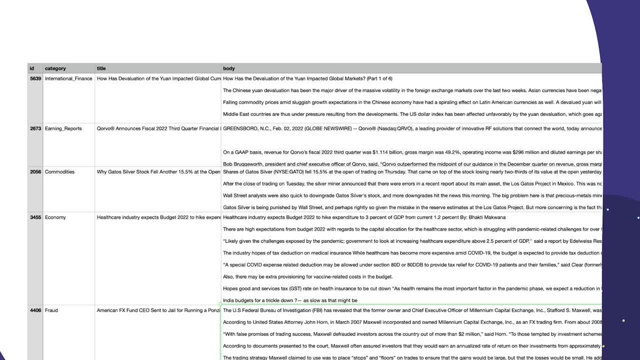 With some code, we should be able to train our AI model to correctly guess what future paragraphs are about. And that's it. Of course, that is a super basic example, and we would need way more data than these 5 paragraphs right here. 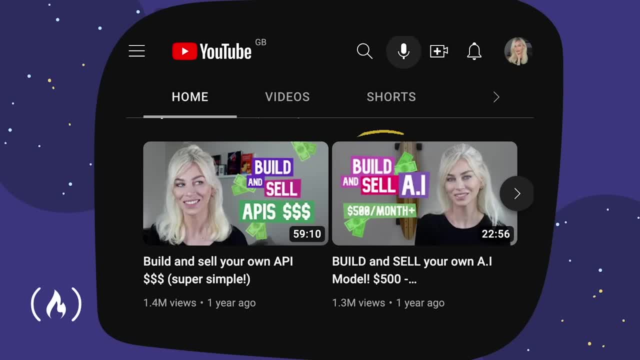 but you get the idea. If you want to build your own AI model and understand the concept of machine learning better as a total beginner, please check out my video on it on my channel Code with Anya Kubo As of now. rapidly improving generative AI techniques can create realistic text responses. 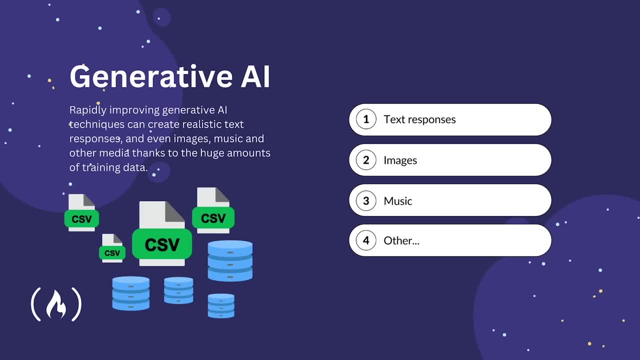 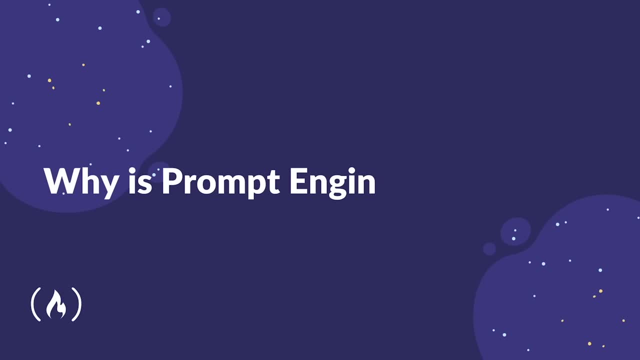 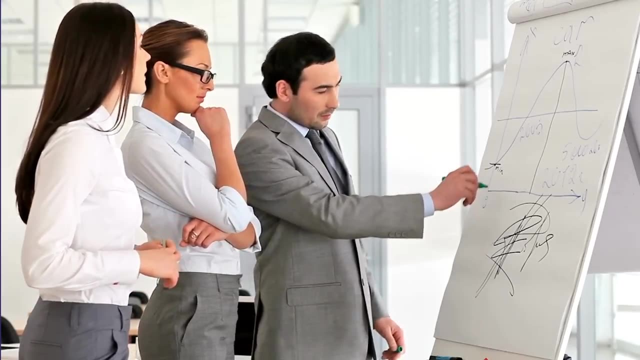 and even images, music and other media, thanks to the huge amounts of training, data and talented developers working on it today. Why is prompt engineering useful? With the quick and exponential growing rise of AI, even the architects of it themselves struggle to control it and its outputs. 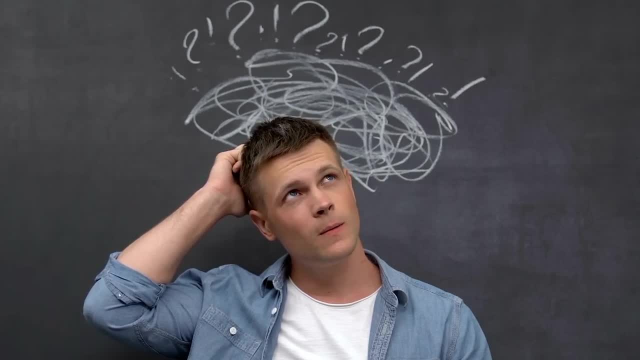 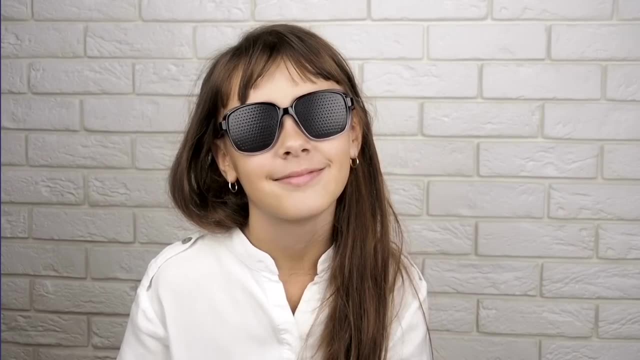 This might be a bit hard to understand, but think of it this way: If you were to ask an AI chatbot what is 4 plus 4, you would expect it to say 8, right, The result of 8 is pretty indisputable. 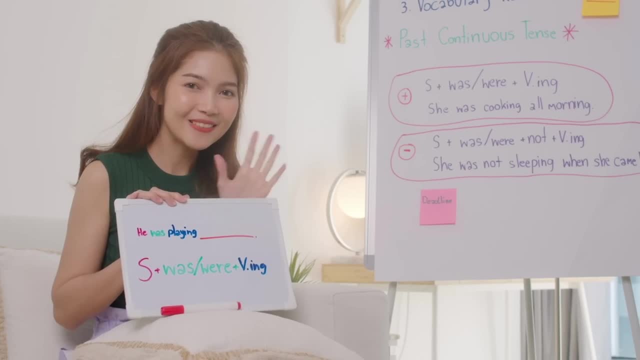 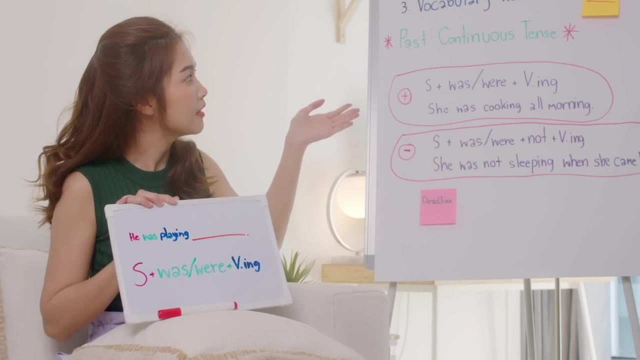 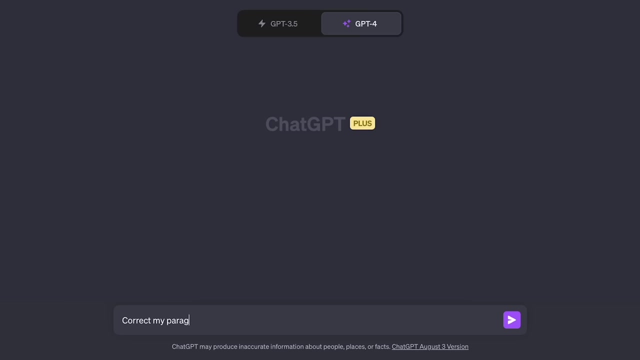 However, imagine you are a young student trying to learn the English language. I'm going to show you how different responses can be based on the prompts you feed and, in turn, your learning experience. For this example, I'm going to be using ChatGPT's GPT-4 model. 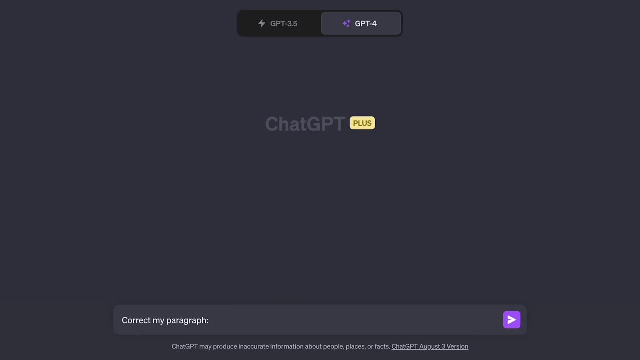 So let's start with the basics. If you were to type correct my paragraph and then pasted a badly written paragraph so just like this, today was great in the world for me. I went to Disneyland with my mom. it could have been better, though, if it wasn't raining. 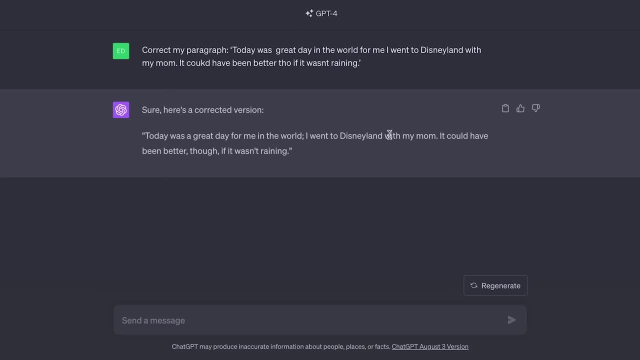 Great. The young English learner has a better sense of the word. But it kind of stops there and the learner is just left to their own devices And, honestly, the sentence really isn't that great anyway. What if the learner could get the best sentences possible from a teacher? 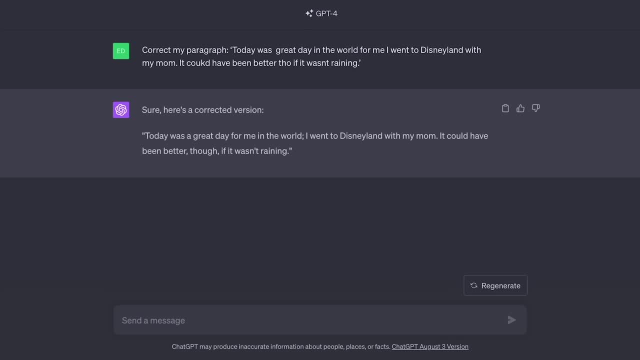 who understands their interests, to keep them engaged With the correct prompts. we can actually create that with AI. So let's give it a go and let's write a prompt to do this. So here's the prompt I'm going to give it. I'm going to write: I want you to act as a spoken. 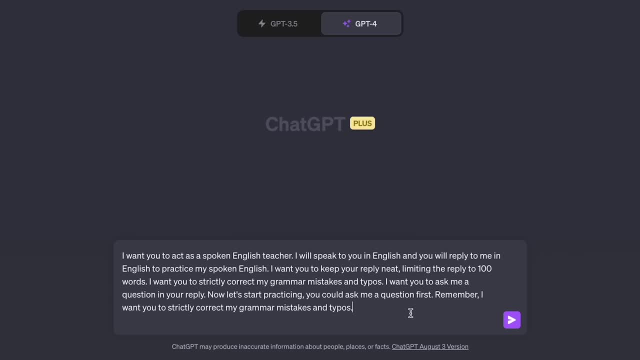 English teacher, I will speak to you in English and you reply to me in English. to practice my spoken English, I want you to keep my reply neat, limiting the reply to 100 words. I also want you to strictly correct my grammar mistakes and typos. 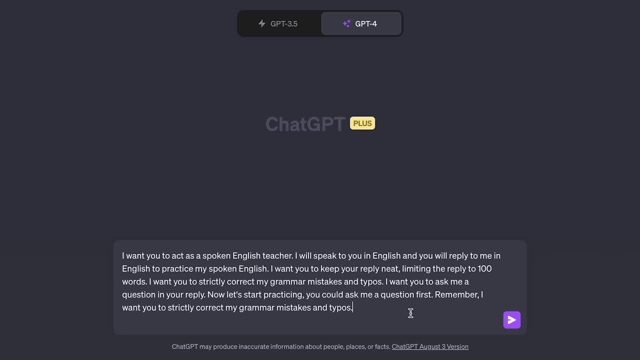 And I want you to ask me a question in your reply. Now, let's start practicing. You could ask me a question first. Remember, I want you to strictly correct my grammar mistakes and typos. So that's my prompt. you can also go a step further and ask it to correct your factual. 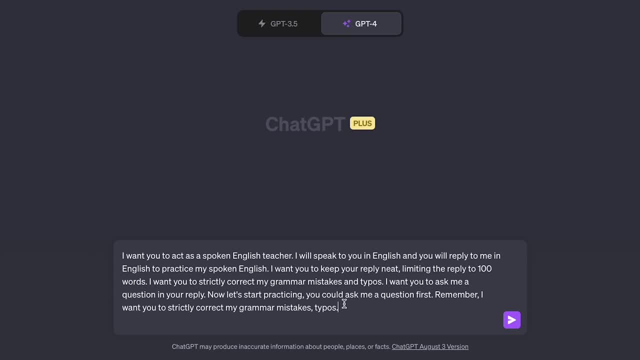 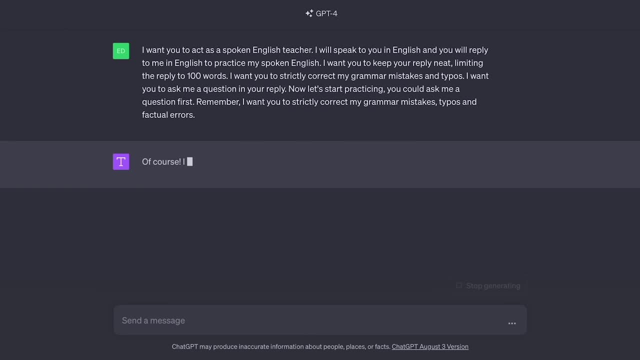 errors too, which I think would be an excellent addition to the prompt. that will benefit the young learner. Okay, so let's go ahead and add that to the prompt. Okay, and let us do its thing, And great. So now this is way more interactive, as you will see- is asking you a question and telling. 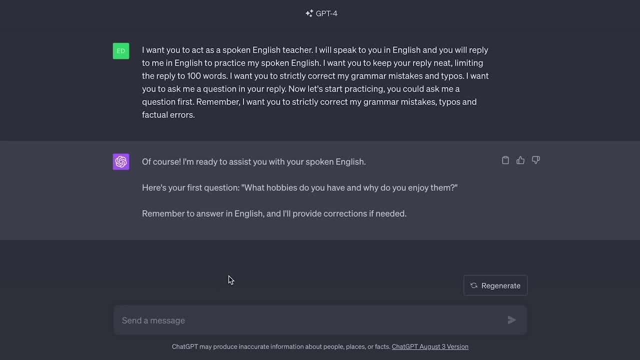 you what to do And we'll provide you with corrections if needed. So, in a way, you're communicating with the AI, it's giving you suggestions and you're learning along the way. it's a completely different experience, Thanks to the prompt that we wrote. Pretty cool, right. 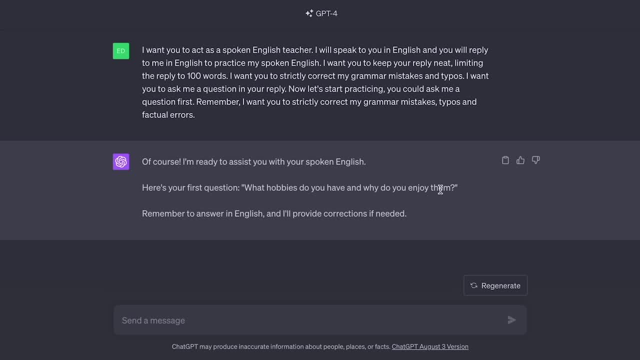 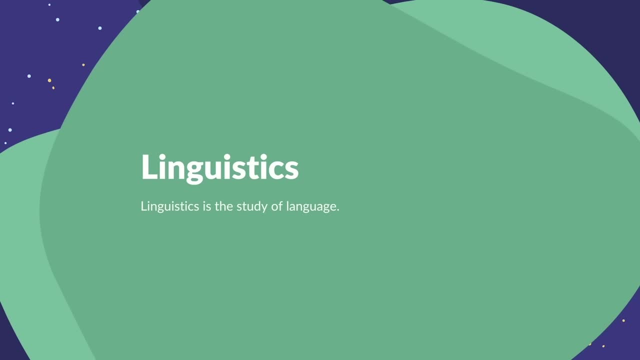 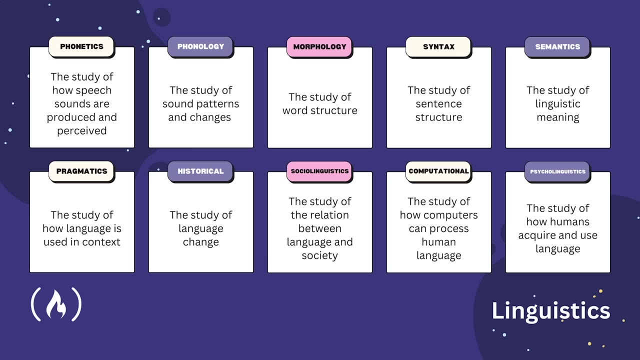 We're going to be diving into a bunch of these concepts soon, But first let's start with the basics: linguistics. linguistics, the study of language. it focuses on everything from phonetics, so the study of how speech sounds are produced and perceived, phonology, So the study of sound. patterns and changes in speech sounds and perceived phonology. So the study of sound patterns and changes in speech sounds and perceived phonology. So the study of sound patterns and changes in speech sounds and perceived phonology. So the study of sound patterns and changes morphology. 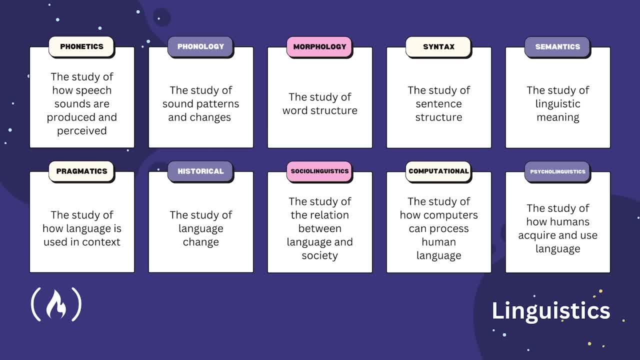 the study of word structure, syntax, so the study of sentence structure. semantics, so the study of linguistic meaning. pragmatics, so in other words, the study of how language is used in context, historical linguistics, or the study of language change, socio linguistics. 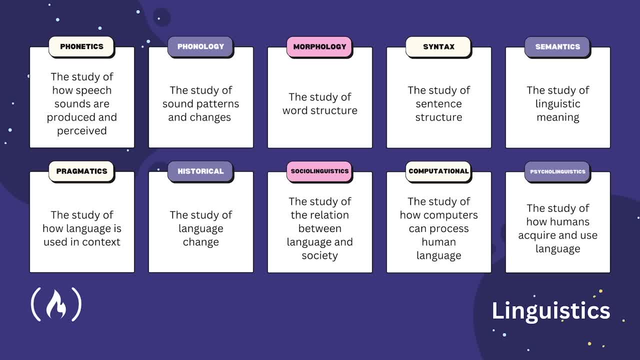 or in other words the study of the relation between language and society, computational linguistics, so the study of how computers can process human language, and physio linguistics, or the study of how humans acquire and use language. So a lot linguistics are the key to prompt engineering. Why? Understanding the nuances? 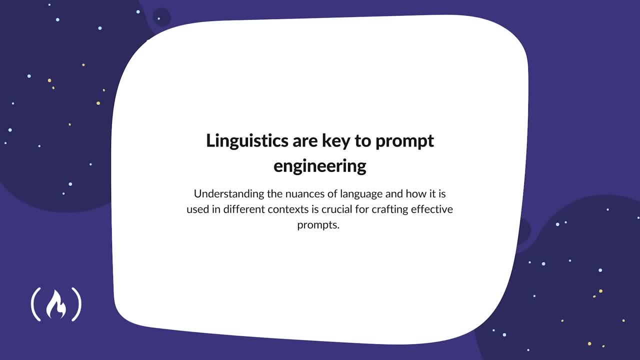 of language and how is used in different contexts is crucial for crafting effective prompts. Not only that, but knowing how to use a grammar or language structure that is universally used will result in the AI system returning back the most accurate results, As you can imagine. 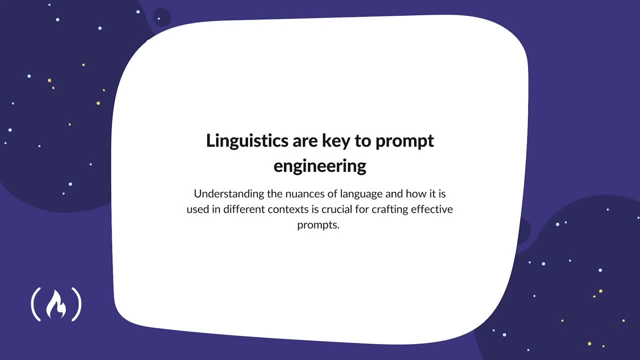 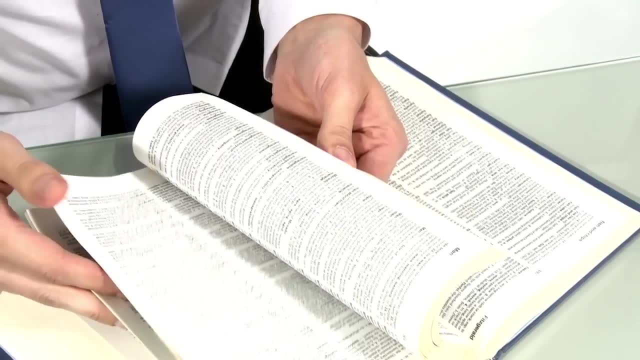 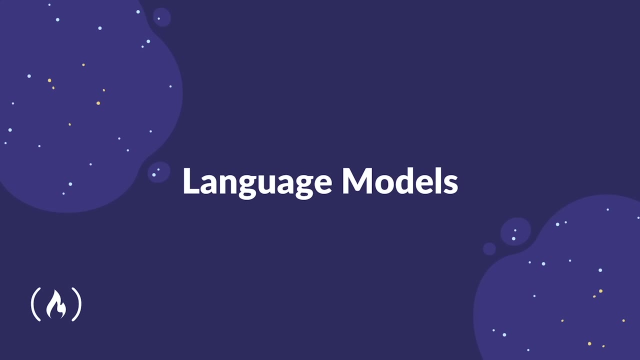 the sheer amount of data that is trained on is most likely to mostly use the standard grammar and language structure that is universally used, So sticking to the standardization is key Language models. Imagine a world where computers possess the power to understand and generate human language, a world where machines can chat, write stories. 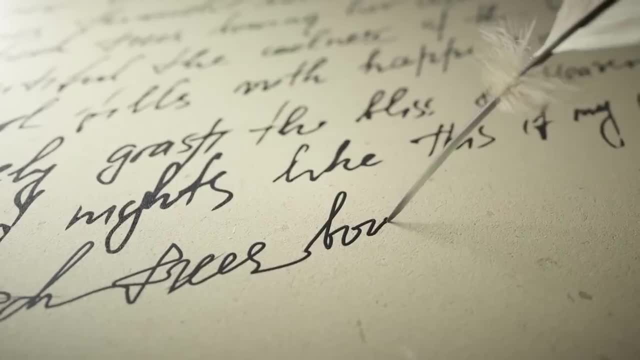 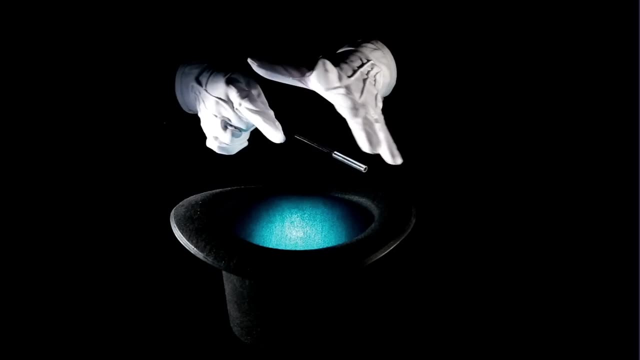 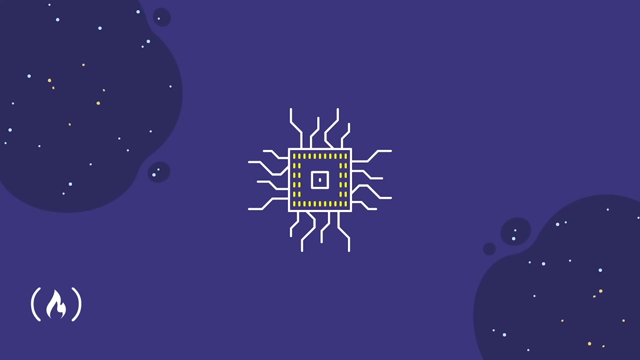 and even compose poetry. In this magical realm, language models can come into play. They are like the wizards of the digital realm, capable of understanding and creating human-like text. A language model is a clever computer program that learns from a vast collection of written text. It takes in books, articles, websites and all sorts of written resources. 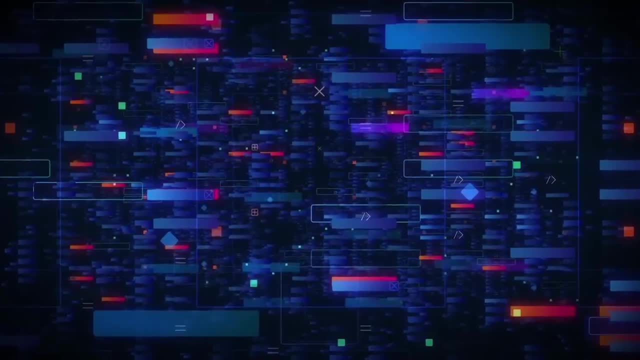 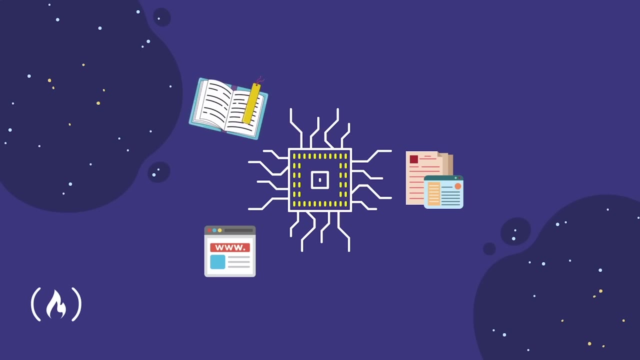 allowing it to gather knowledge about how humans use language. Just like a master linguist, it becomes an expert in the art of conversation, grammar and style. But how does this all work? Well, imagine you feed a sentence. The language model will then analyze the sentence. 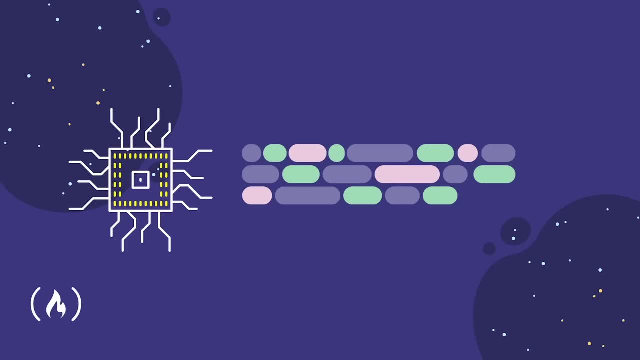 examine the order of words, their meanings and the way they fit together, Then the language model will generate a prediction or a continuation of the sentence that makes sense. based on its understanding of the language, It will weave words together one by one, creating a response. 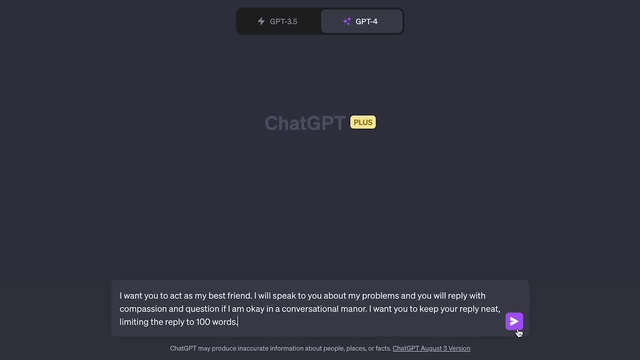 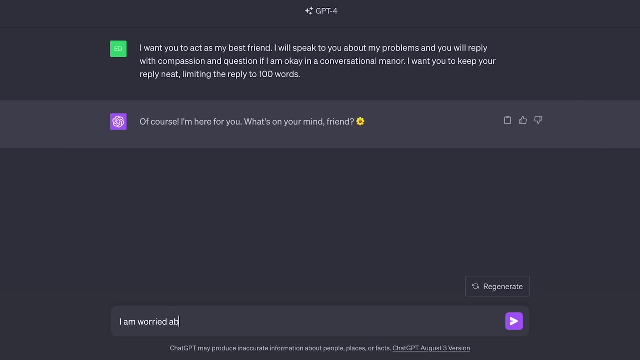 that seems like it was crafted by a human being. Imagine having a conversation with the language model, as if you were exchanging ideas with a digital friend. You ask a question and it responds with a well-crafted answer. You tell a joke. 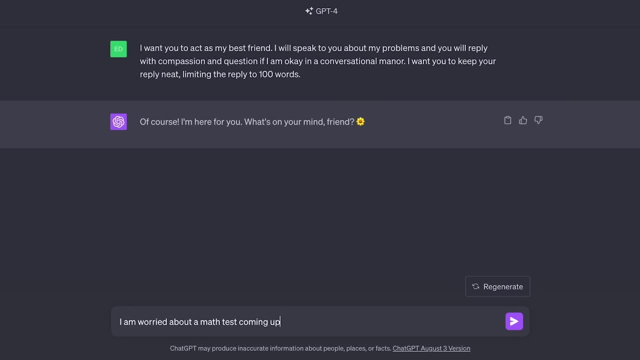 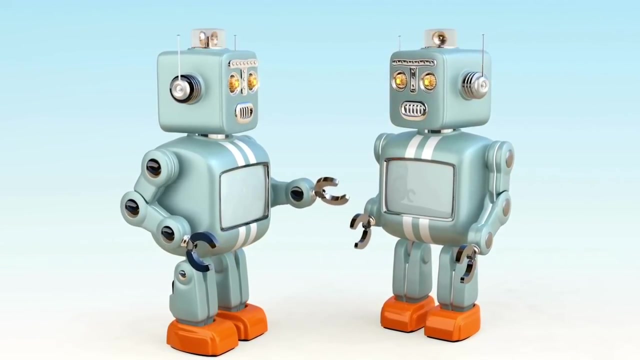 and it counters with a witty remark: It's like having a language expert by your side, always ready to assist and engage in conversation. Now you may wonder where these language models are used. They can be found in various places, from your smartphone's virtual assistants to customer service chatbots, and even in the 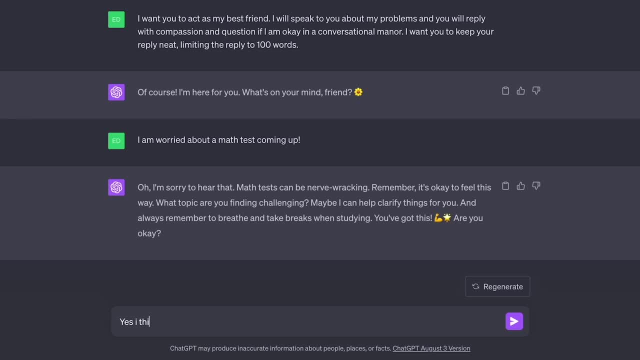 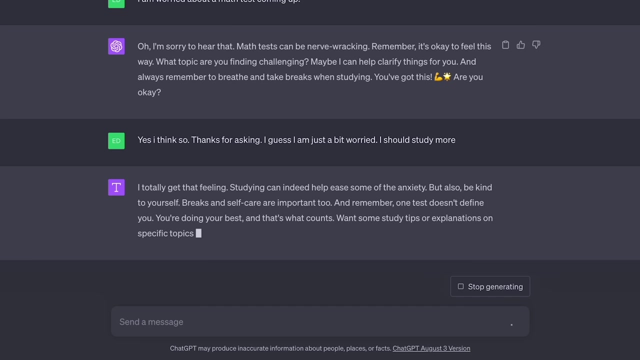 creative realm of writing. They help us find information, offer suggestions and create content. But remember, while language models possess incredible abilities, they still rely on the humans who create and train them. They are, in fact, a fusion of human ingenuity and the power. 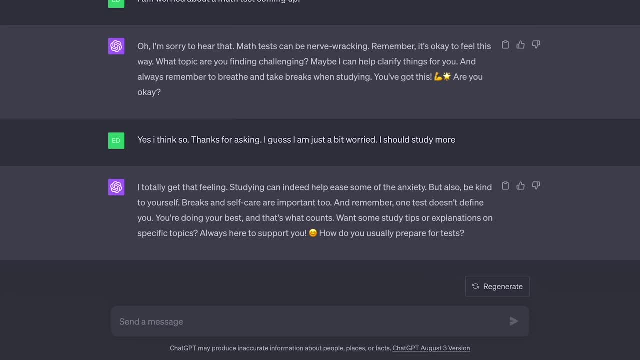 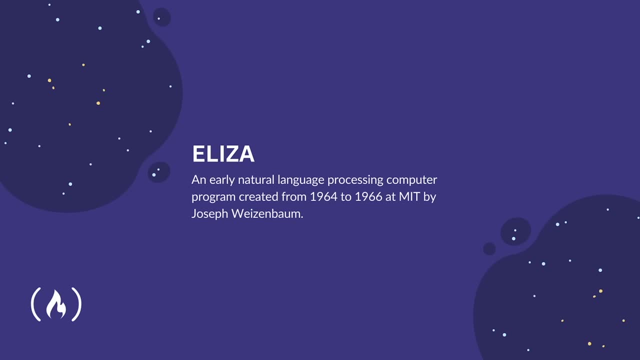 of algorithms, blending the best of both worlds. Let's start off by looking at the history of language models, starting with the first AI ELISA back in the 60s. ELISA is an early natural language processing computer program created from 1964 to 1966 at MIT. 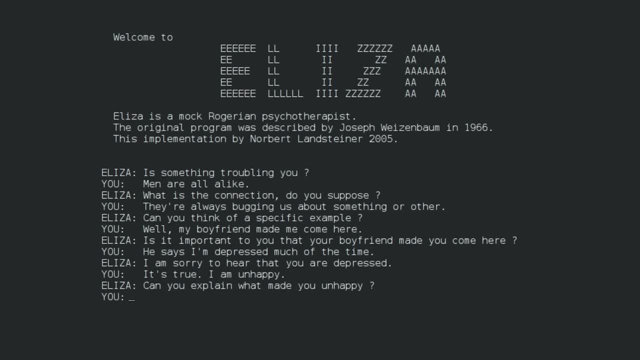 Wiesenbaum. ELISA was designed to simulate a conversation with a human being. ELISA had a special knack for mimicking a Rogerian psychotherapist, someone who essentially listens attentively and asks probing questions to help people explore their thoughts and feelings. 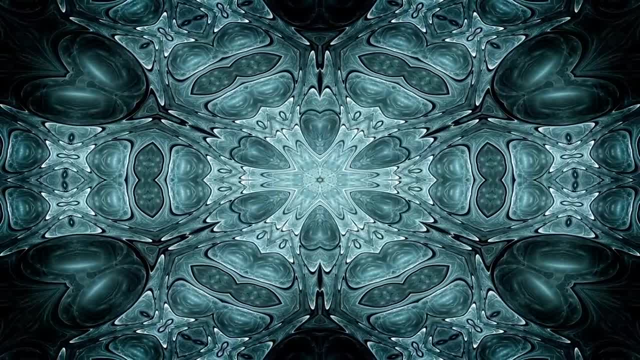 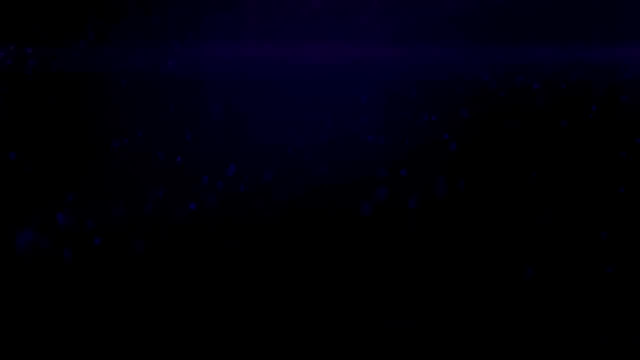 ELISA's secret weapon was its mastery of pattern matching. It had a treasure trove of predefined patterns, each associated with specific responses. These patterns were like magical spells that allowed ELISA to create a new world for itself. ELISA's secret weapon was its mastery of pattern. matching. It had a treasure trove of predefined patterns, each associated with specific responses. ELISA's secret weapon was its mastery of pattern matching. It had a treasure trove of predefined patterns, each associated with specific responses. ELISA's secret weapon was its mastery of pattern. 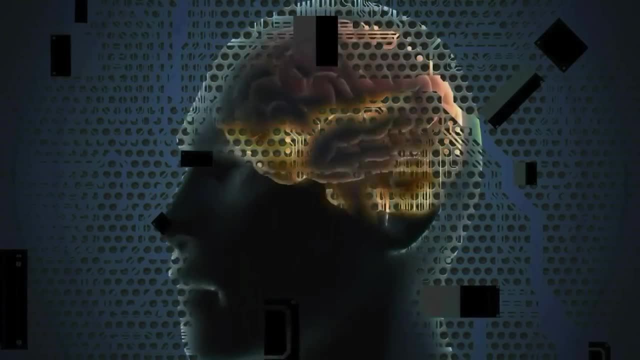 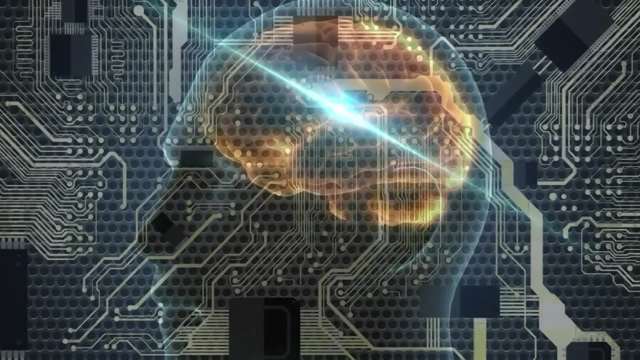 matching. It had a treasure trove of predefined patterns, each associated with specific responses. When you engaged in a conversation with ELISA, it would carefully analyze your input, seeking patterns and keywords. It would then transform your words into a series of symbols. 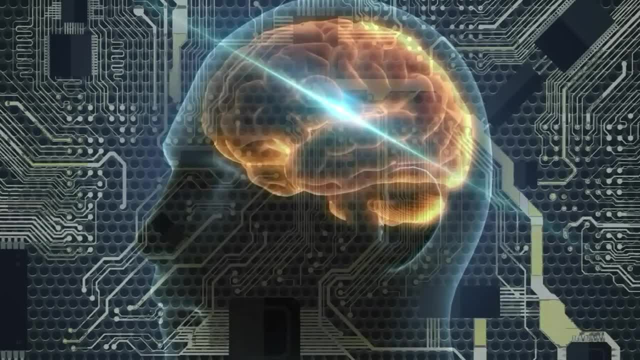 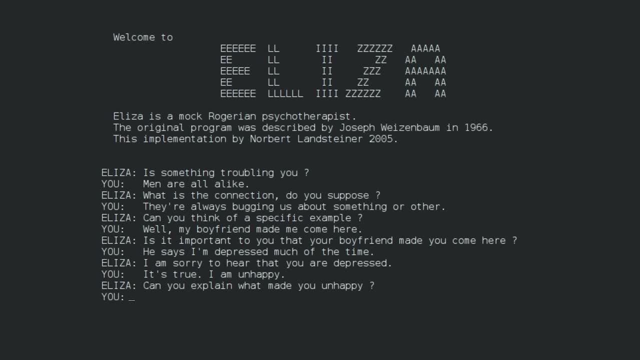 searching for patterns that matched those symbols in its repertoire. Once a pattern was detected, ELISA would work its magic by transforming your words into a question or statement that aimed to explore your thoughts and emotions. It was as if ELISA was holding up a metaphorical mirror. 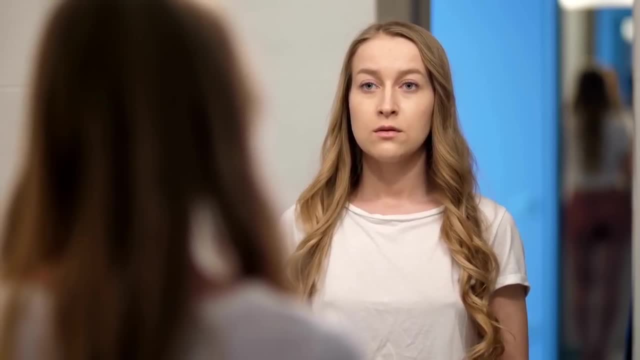 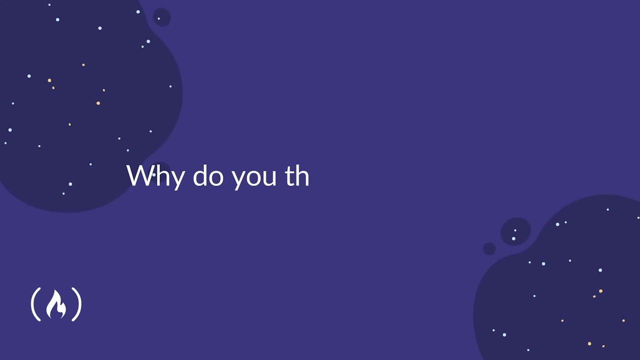 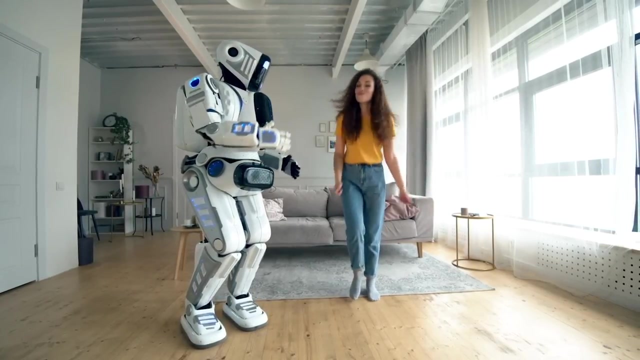 encouraging you to delve deeper into your own thinking. For example, if you said something like I feel sad, Eliza would detect the pattern and respond with a question like: why do you think you feel sad? It encouraged reflection and introspection, just like a caring therapist would. 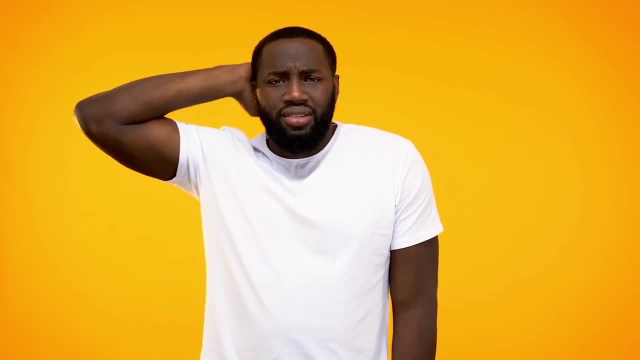 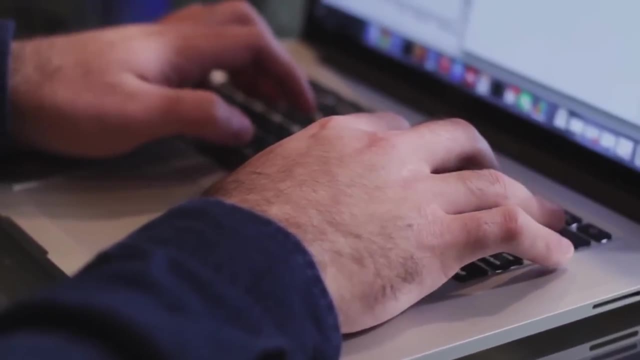 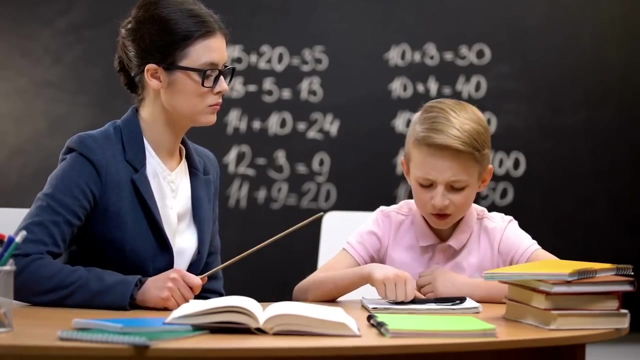 But here's the delightful twist: Eliza didn't truly understand what you were saying. It was just a clever illusion. It used pattern matching and some creative programming tricks to create the illusion of understanding, while in reality it was just following a set of predefined rules. 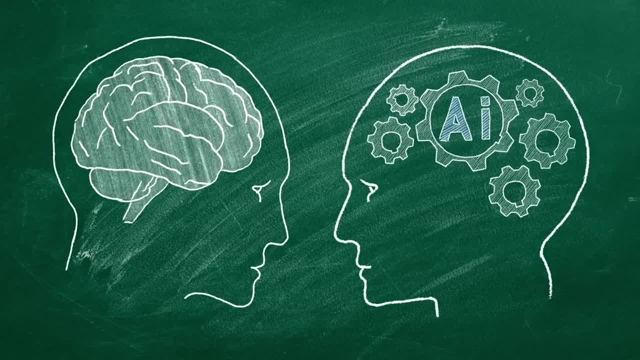 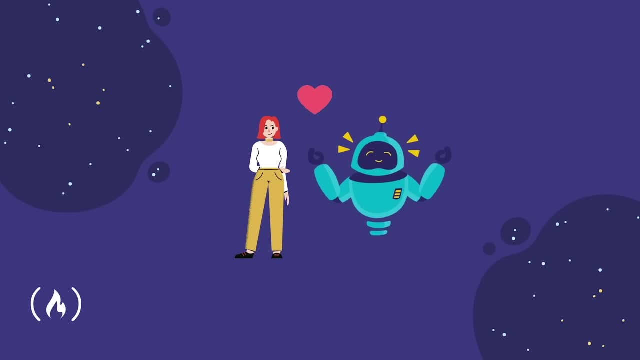 Yet even though Eliza was a simple program, people were often captivated by its conversational abilities. They felt heard and understood, even if they knew they were talking to a machine. It was like having a digital confident who was always ready to listen and offer gentle guidance. 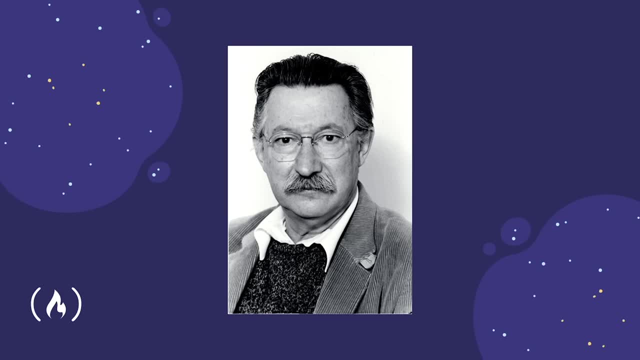 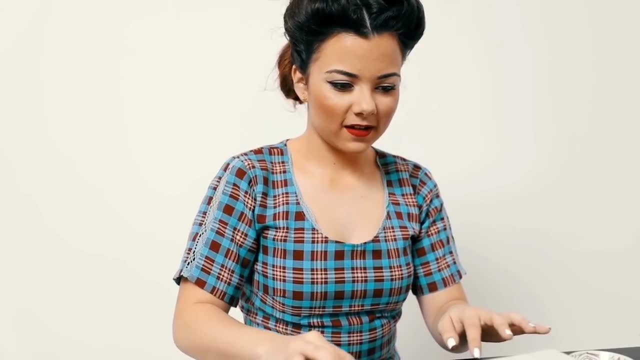 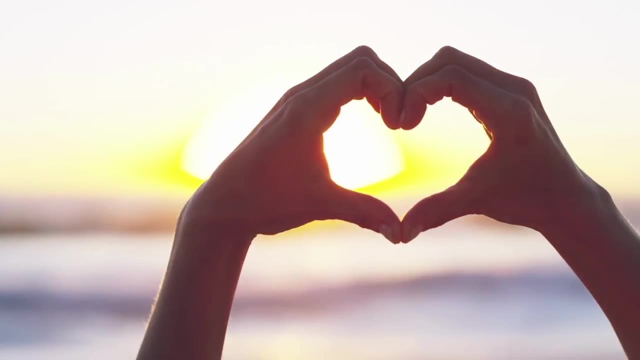 Eliza's creator, Weizenbaum, intended the program as a method to explore communication between humans and machines. He was surprised and shocked that individuals, including his secretary, attributed human-like feelings to the computer program. But that is a whole other topic of conversation in itself. 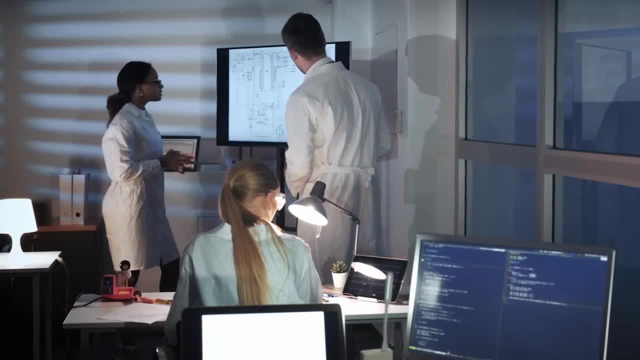 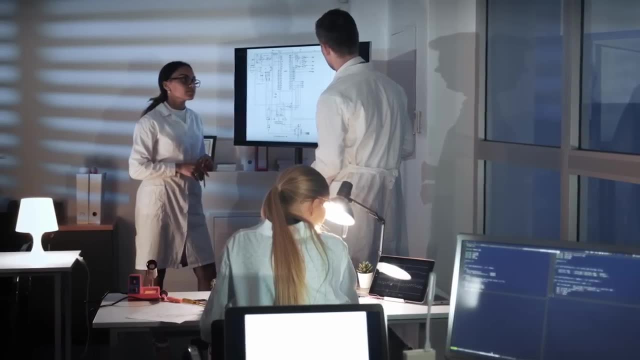 Eliza's impact was profound, sparking interest and research in the field of natural language processing. It paved the way for more advanced systems that could truly understand and generate human language. It was the humble beginning of a grand adventure in the world of conversational AI. 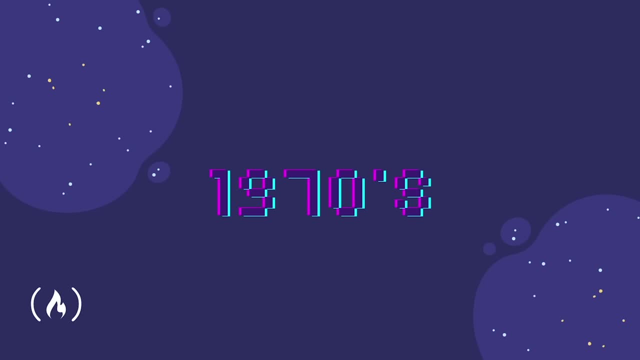 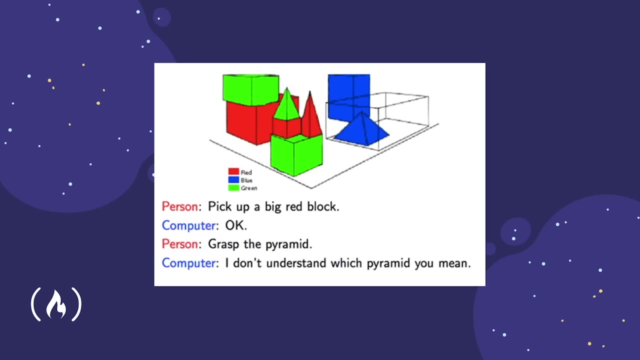 Fast forward to the 1970s, when a program named SHRDLU appeared. It could understand simple commands and interact with a virtual world of blocks. Although SHRDLU wasn't a language model per se, it laid the foundation for the idea of machines comprehending human language. 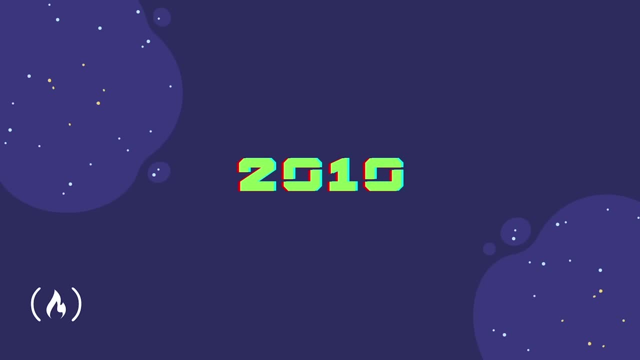 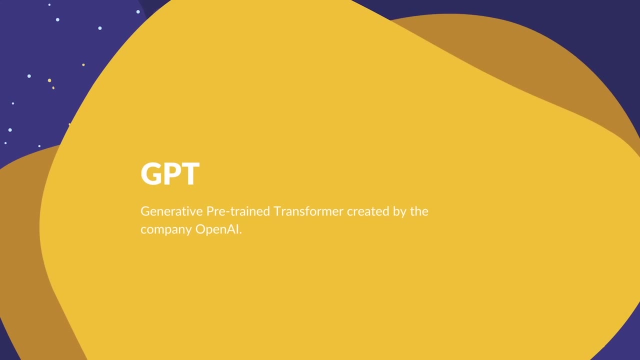 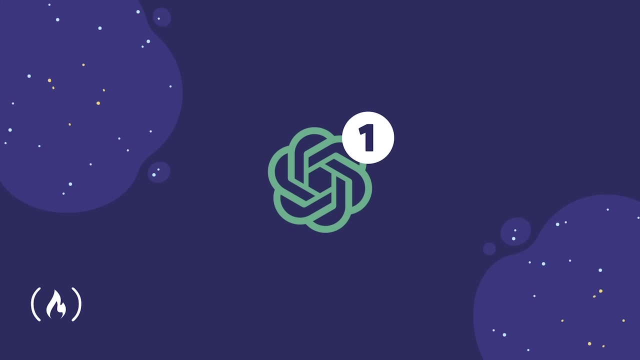 But the true language models began around 2010,, when the power of deep learning and neural networks came into play. Enter the mighty GPT, short for Generative Pre-trained Transformer, ready to conquer the world of language. In the year 2018, the first iteration of GPT emerged, created by the company OpenAI. 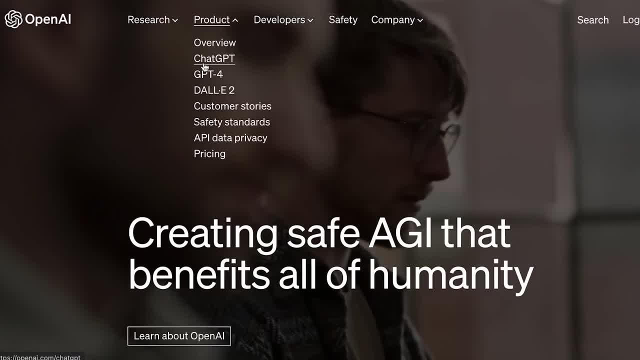 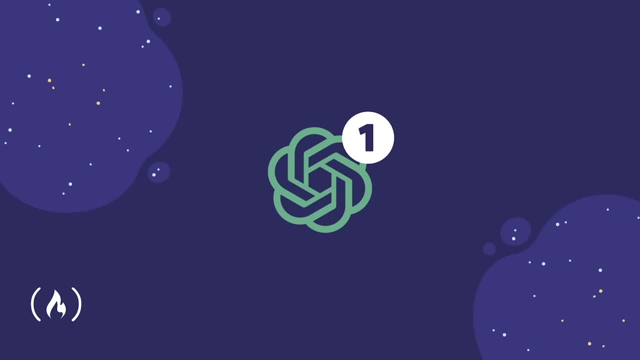 It was trained on a large amount of text data, absorbing knowledge from books, articles and a large chunk of the internet. GPT-1 was a taste of things to come, an impressive language model, but small compared to its descendants that we use today. 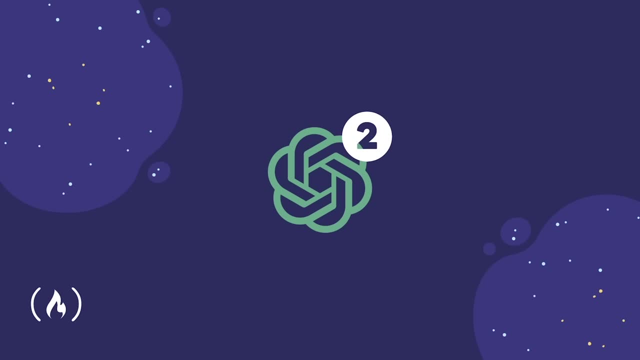 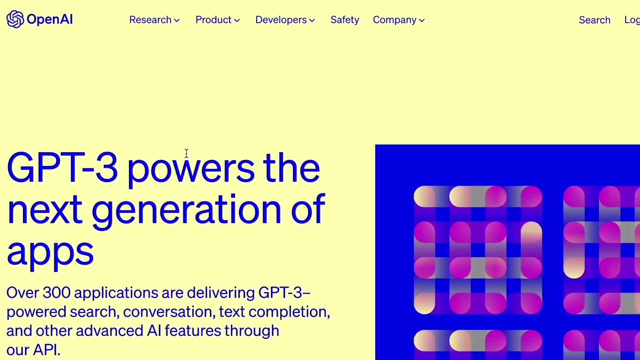 As time went on, the saga continued with the arrival of GPT-2 in 2019, followed by GPT-3 in 2020.. This was a titan among language models, equipped with a large number of parameters- over 175 billion to be precise. 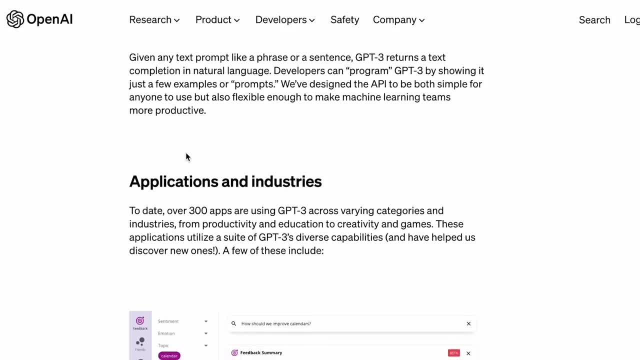 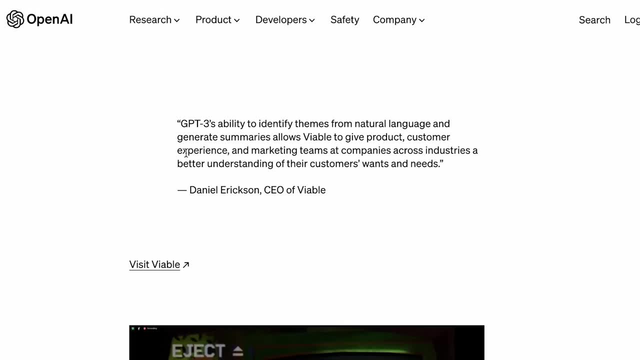 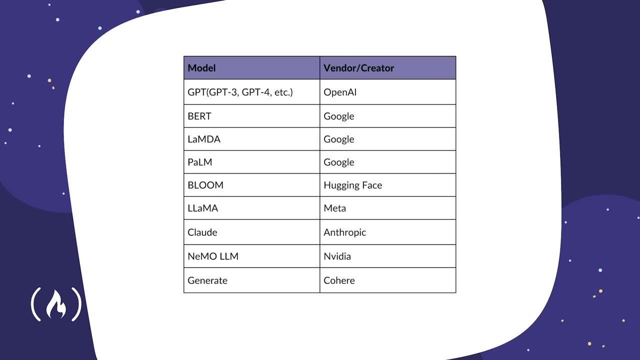 GPT-3 dazzled the world with its unparalleled ability to understand, respond and even generate creative pieces of writing. The arrival of GPT-3 marked a real turning point in terms of language models and AI At the time of writing. we now also have GPT-4, trained on pretty much the whole internet. 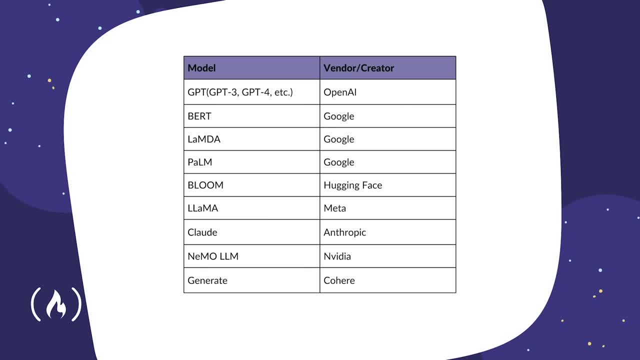 rather than outdated large data sets, as well as BERT from Google and so much more. It would seem we are only just at the start when it comes to language models and AI, so learning how to harness this data with prompt engineering is a smart move for anyone today. 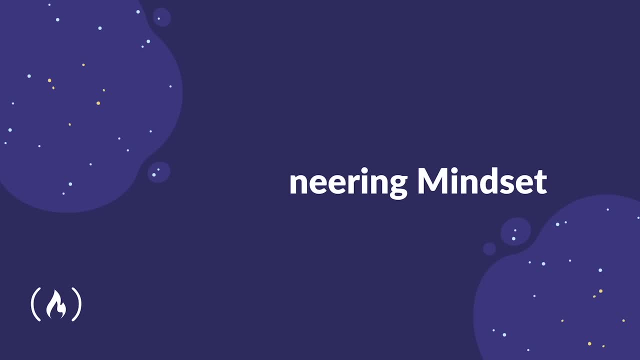 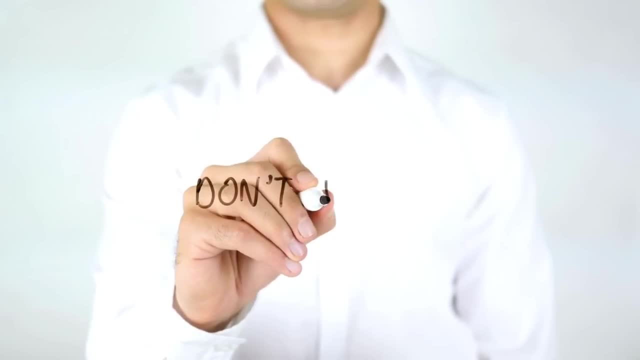 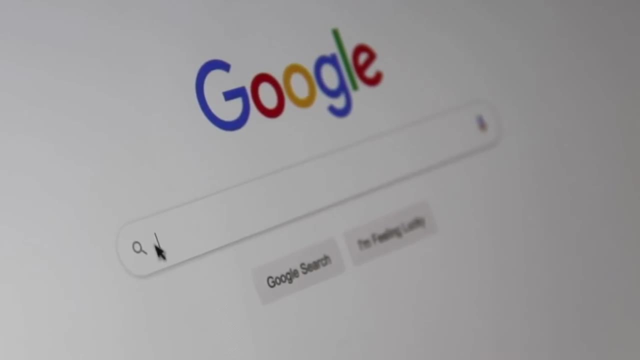 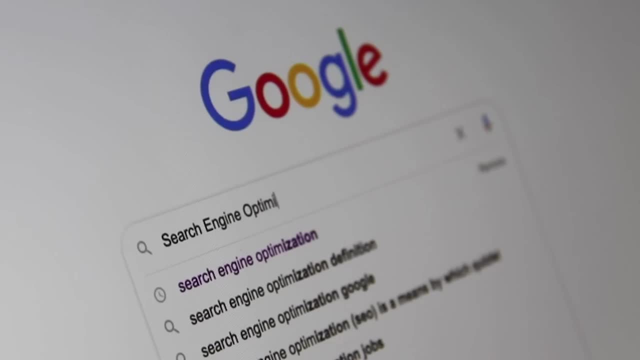 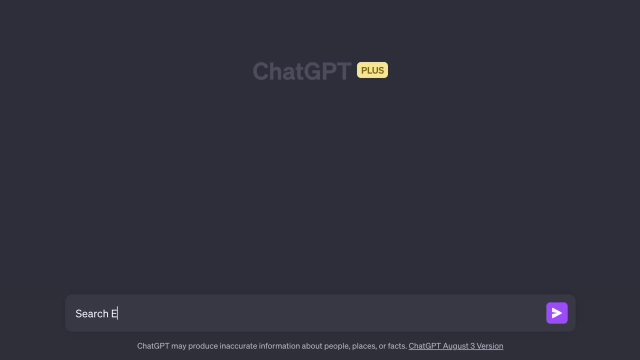 skills now, as opposed to five years ago, I'm assuming, a lot better. We have grown to intuitively know what to type into Google the first time round as to not waste time. Having the same mindset for prompt engineering can also be applied. In conclusion, if you want to learn more about Google, check out the full video on the website. 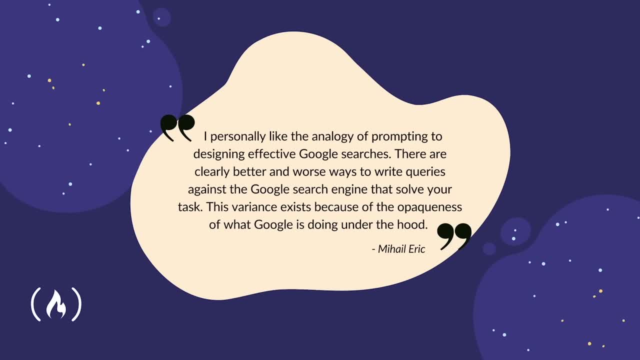 and I will see you in the next video. Bye. Mihail Erick of the Infinite Machine Learning podcast says it well when he says: I personally like the analogy of prompting to designing effective Google searches. There are clearly better and worse ways to write queries against the Google search engine. 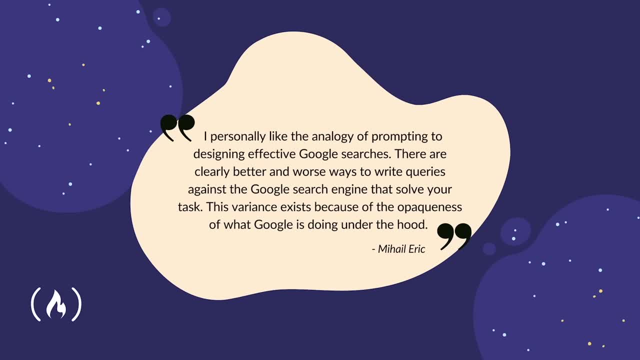 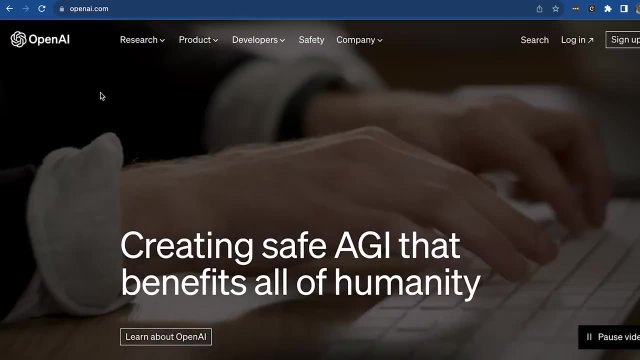 that solve your task. This variance exists because of the opaqueness of what Google is doing under the hood. We are going to keep this in mind for the remainder of the course. A quick intro to using ChatGPT by OpenAI. So, as I said in this course, for the examples I will be using ChatGPT's GPT-4 model. 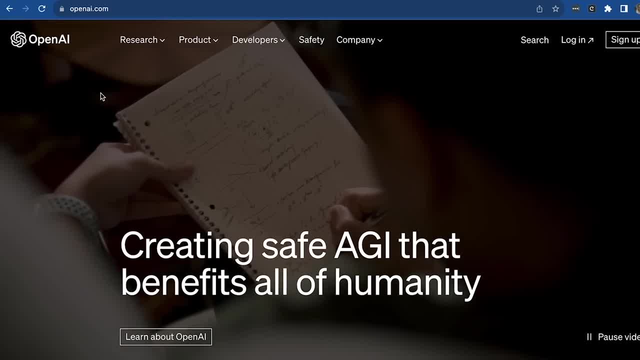 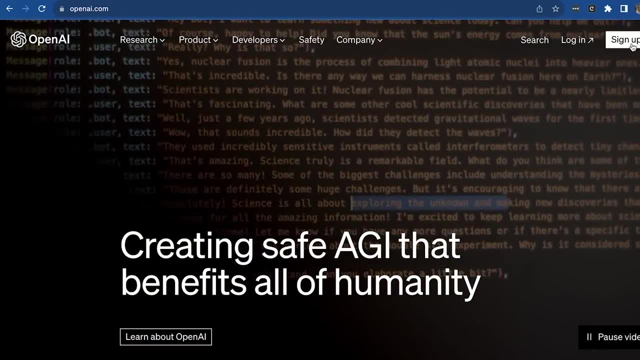 In order to follow along or just to understand how we are going to be using the platform, please head over to OpenAIcom and just go ahead and sign up. I've already signed up, so I'm just going to go ahead and log in. 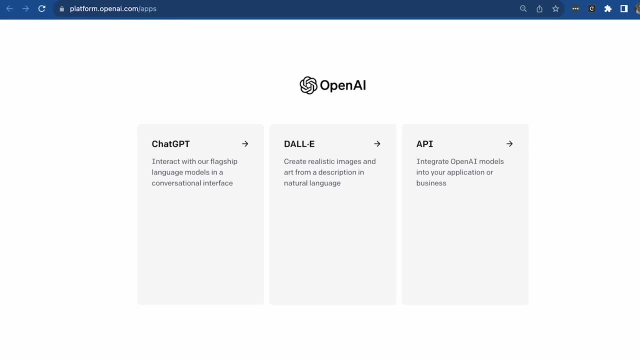 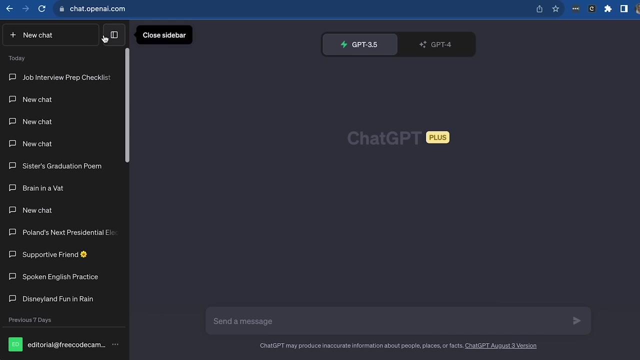 And that will take me to the platform in which I can choose what I want to interact with. For this tutorial, we are going to be interacting with ChatGPT-4.. So please go ahead and click on here, And that will take you to the platform. 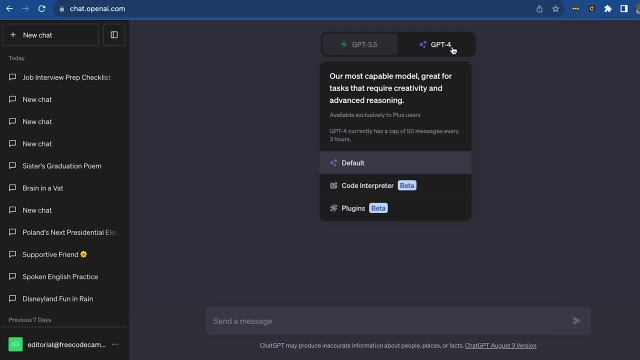 And then I'm just going to go ahead and switch to the GPT-4 model, which is the latest one. Okay, so great. You will see here all the previous chats that I've had. I'm just going to minimize this. 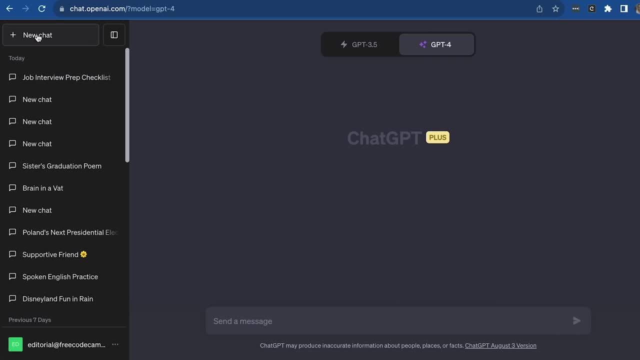 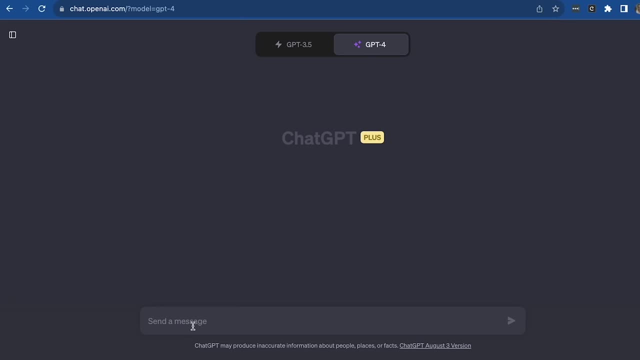 And if we want to create a new chat, all we'd have to do is click the new chat button. Okay, so here, for example, what I can do is just go ahead and ask any questions. So what is 4 plus 4?? 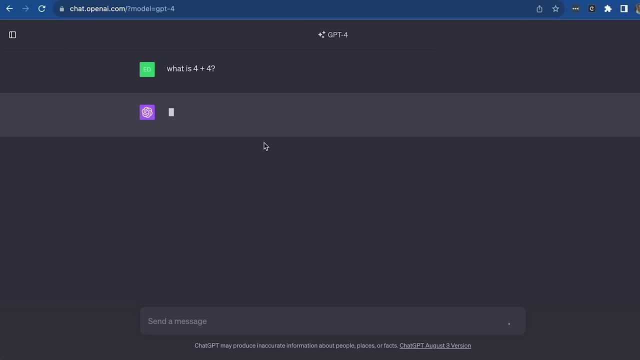 And then hit send And that will essentially give me a response. So I'm now interacting with ChatGPT-4.. On this occasion I can actually build on the previous conversation, So what I can do is say: great, Now can you ask? 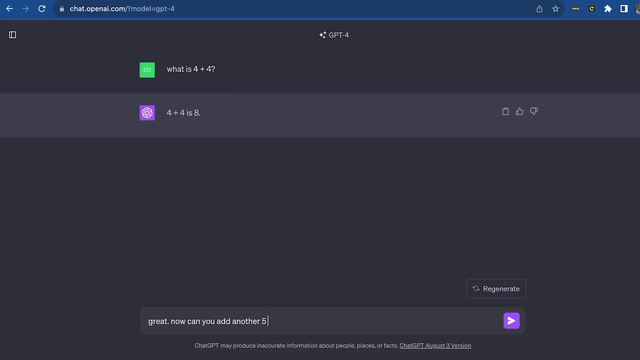 Can you add another 5 to that? What is the answer? And it will take into account everything that I have previously. Okay, I am building on top of the knowledge that it already has. Great. So, again, this is just a very quick introduction to how to use this. 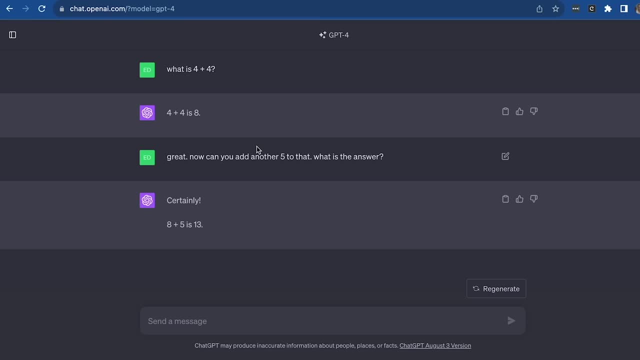 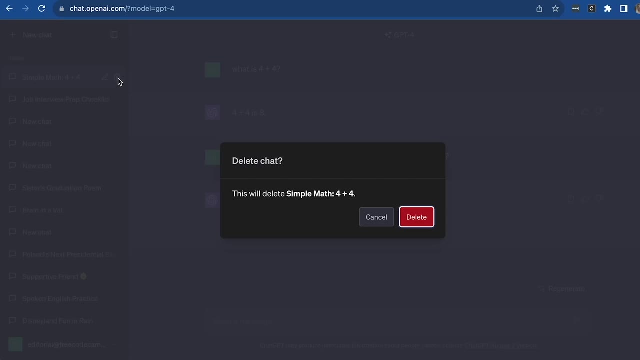 We will be doing a deeper dive into this throughout this course. So, once again, to create a new chat, we're going to click on here. All you'd have to do is create new chat And if you want to delete the old one, just go ahead and click that delete button. 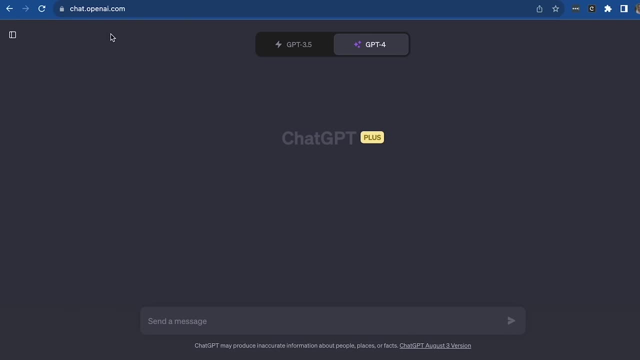 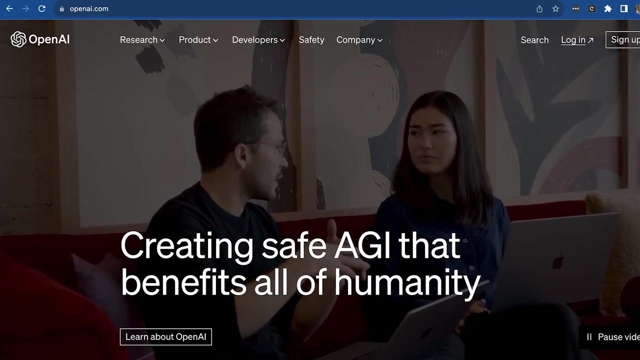 And that will delete it, And then a new chat is brought up automatically. Wonderful. Now you might have seen my course on OpenAI, in which we can also use the API. And to use the API, just go over to the API references. 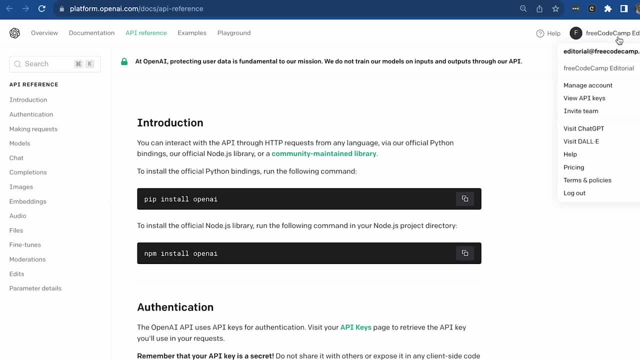 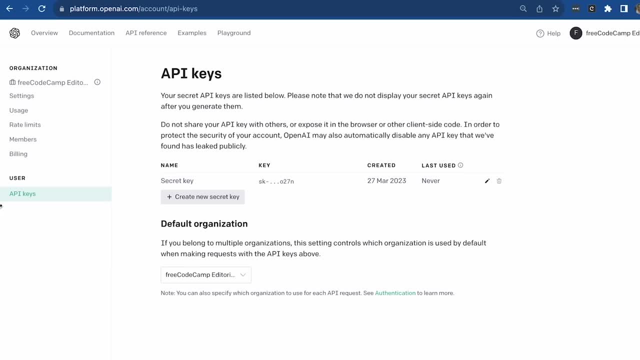 And all you would have to do is get an API key And the API key can be viewed, And then you just go ahead and create an API key, And that will allow you to interact with the OpenAI API in order for you to build out your own platforms. 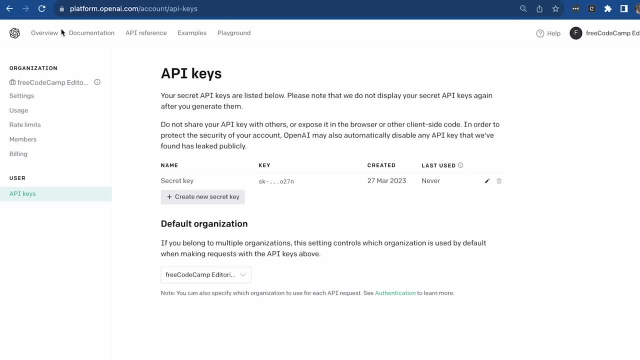 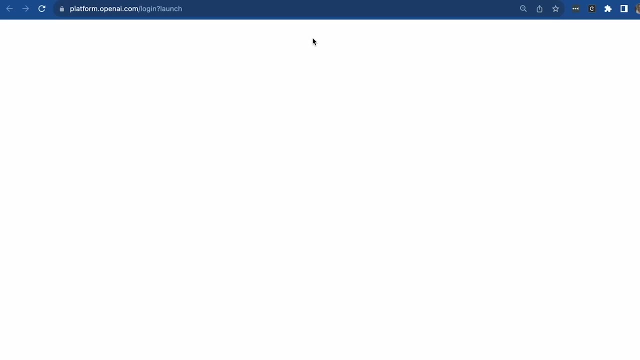 just as the one we saw before. So if you're interested in that, please do head over to my tutorial on this, again on the free CodeCamp channel. Otherwise, let's continue using ChatGPT. So once again, I'm just going to log in and head back to the platform. 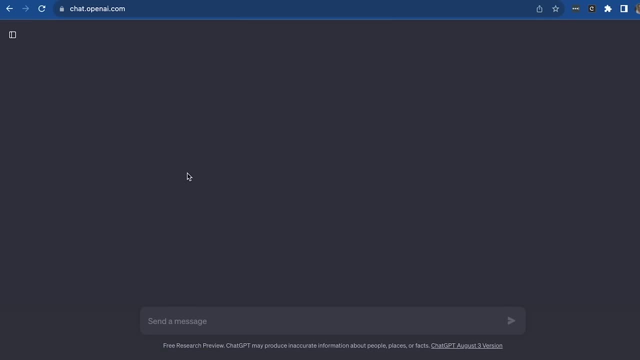 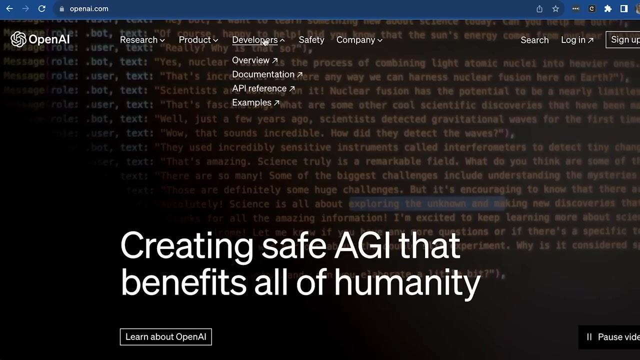 Here we go, And that is it. we are ready to go. Another thing I want to discuss is tokens, as you might find that you have run out of the free tokens that you have in order to interact with ChatGPT, So in order to do that, I'm just going to show you this. I'm going to head over to the documentation. 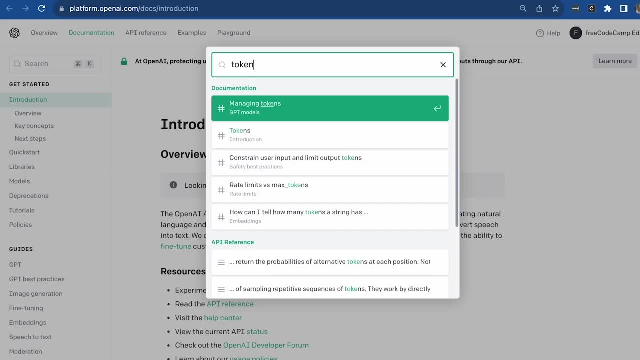 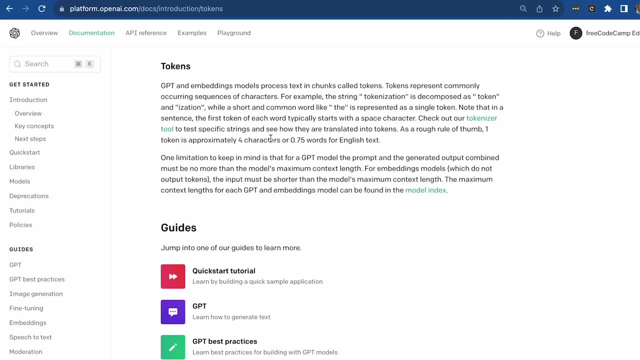 and talk to you a little bit about tokens. So GPT-4 essentially processes- It's all text in chunks called tokens, And this token is approximately four characters or 0.75 words for English text, And we essentially get charged by token. 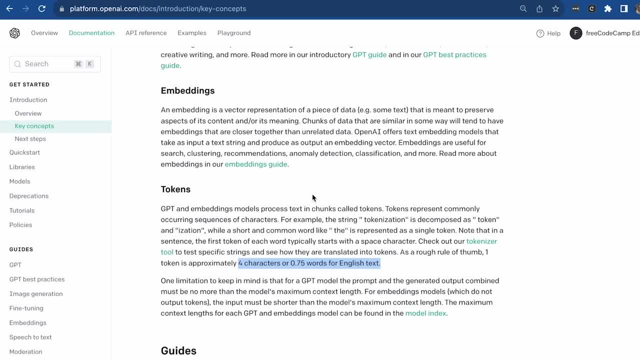 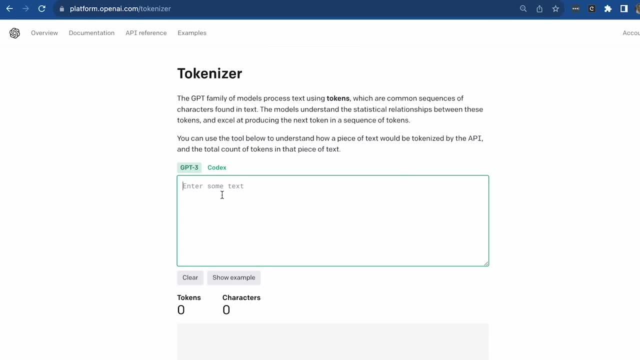 If you want to know exactly how many tokens you are using, you can check it out here. You can check out the tokenizer tool and it will give you a rough example. So, for example, I can say what is tokenized: It is four plus four. 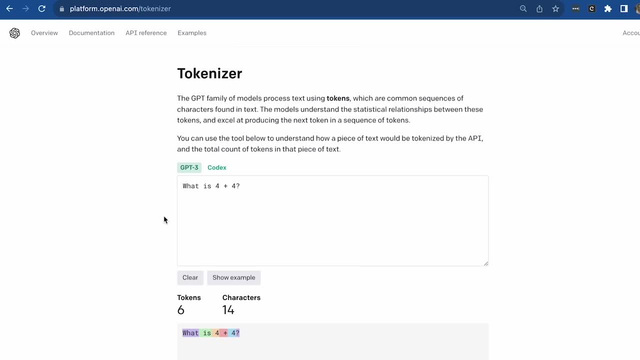 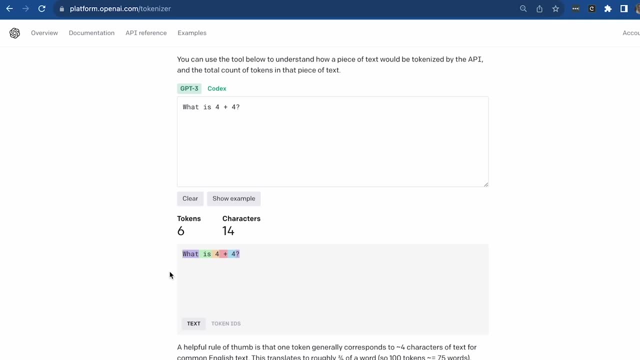 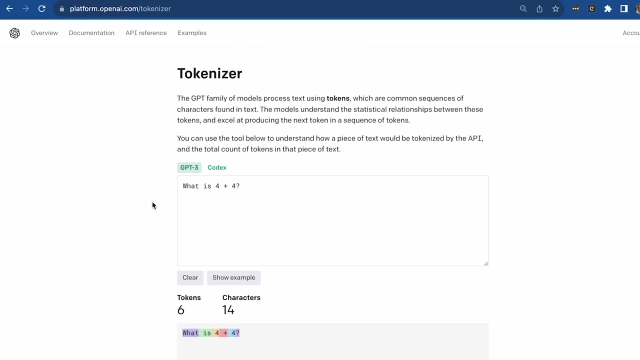 And with that piece of text, the total count of tokens is going to be six. Okay, so there we go. That is exactly how many tokens will be used in order to produce a answer for this request. Great, So here is the URL for that. you can play around with it. 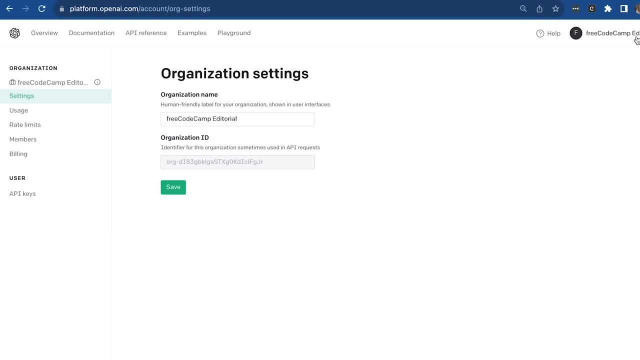 I hope you have fun. If you want to see your usage, you can head over to your account And then You can manage your account and this should be able to show you your usage. So it will show you your usage right here per month. 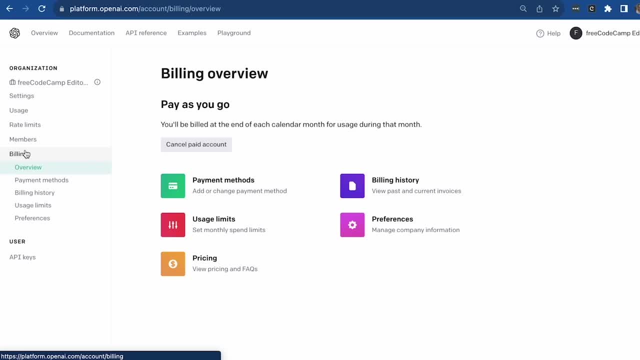 And then you can of course, also add billing in order to carry on using chat GPT, in case you use up all your tokens and you can't use it anymore. So once again, this is under account billing overview, So just go check it out. 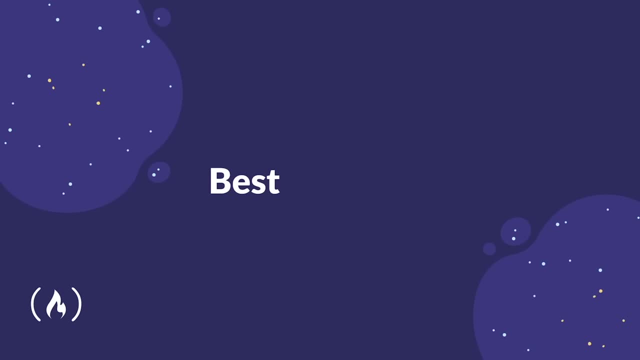 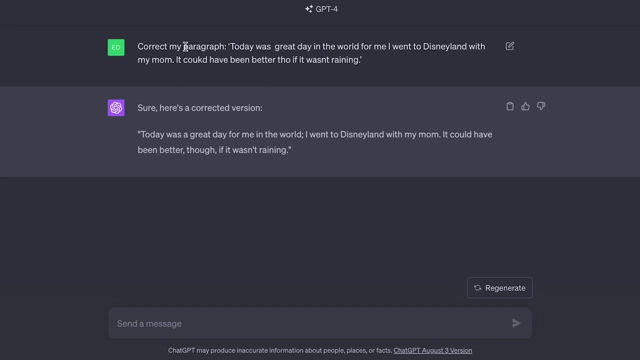 Okay, And now back to the platform Best practices. The biggest misconception when it comes to prompt engineering is that it's an easy job with no science to it. I imagine a lot of people think it's just about constructing a one off sentence, such as correct my paragraph that we saw in the previous example. 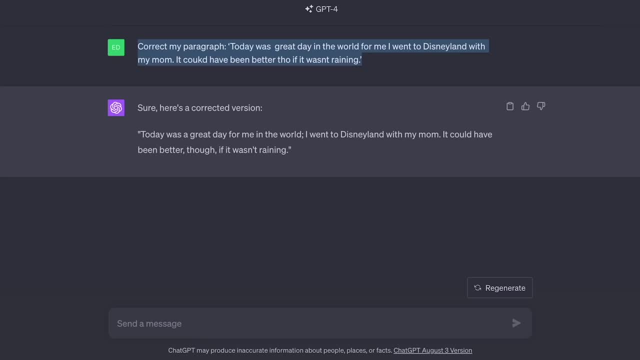 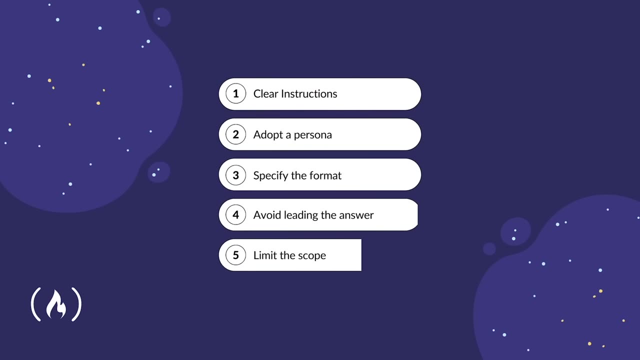 When you start to look at it. creating effective prompts relies on a bunch of different factors. Here are some things to consider when writing a good prompt: Consider writing clear instructions With details in your query. consider adopting a persona as well as specifying the format using iterative prompting, meaning if you have a multi part question or if the first response wasn't sufficient, you can continue by asking follow up questions or asking the model to elaborate and avoid leading the answer. 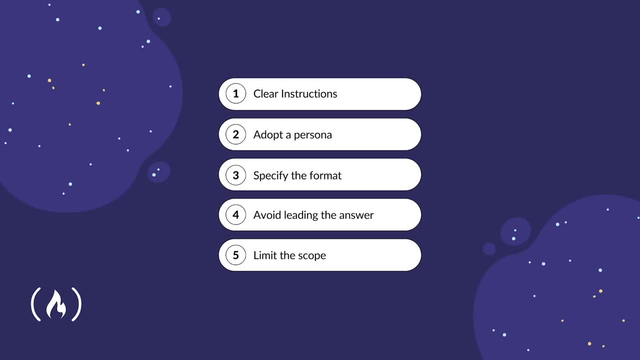 Try not to make your prompt so leading that it inadvertently tells the model what answer you're expecting. This might bias the response on Julie And, finally, limit the scope for long topics. If you're asking about a broad topic, it's helpful to break it down or limit the scope to get a more focused answer. 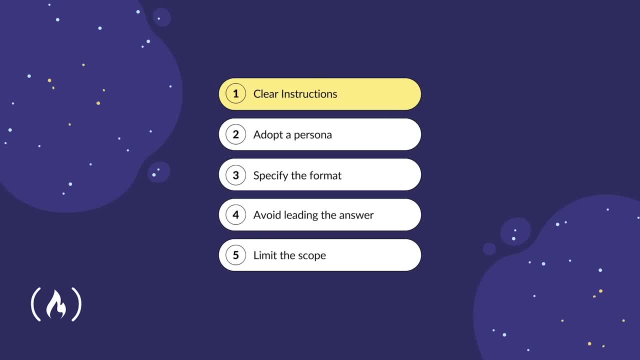 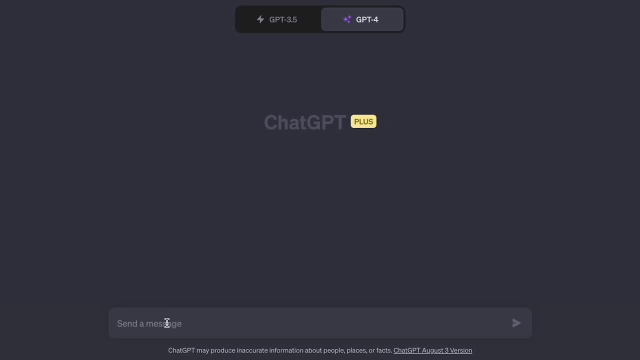 Let's look at some of these now. In order to write clearer instructions, we can adopt writing more details in our queries and to get the best results. Don't assume the AI knows what you are talking about. Writing something like when is the election implies that you are expecting the AI to know what election you are talking about. 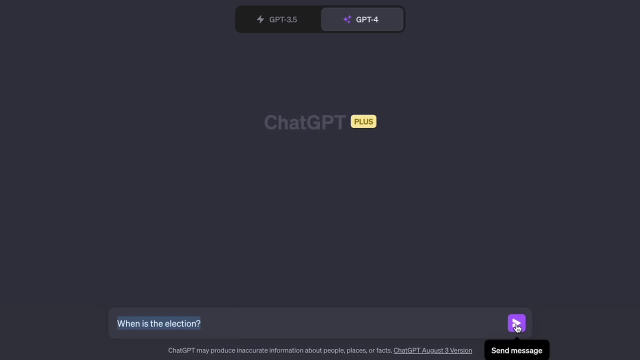 And what country you mean. This may result in you asking a few follow up questions to finally get the result you want, resulting in time loss and, frankly, perhaps some frustration. Consider taking the time to write a prompt with clear instructions So, for example, instead of writing when is the election, you could write when is the next presidential election for Poland? 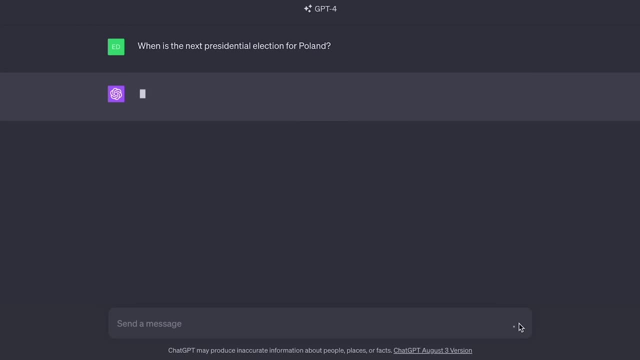 So let's go ahead and run this, And this will be much more precise. And this will be much more precise And this will be much more precise. It knows exactly what we are asking about. It's not going to go guessing and waste our time, as well as waste our resources. 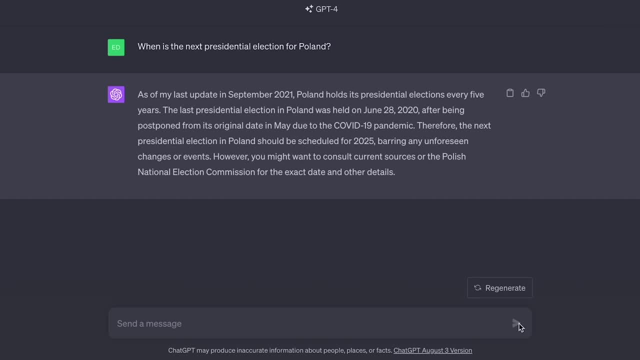 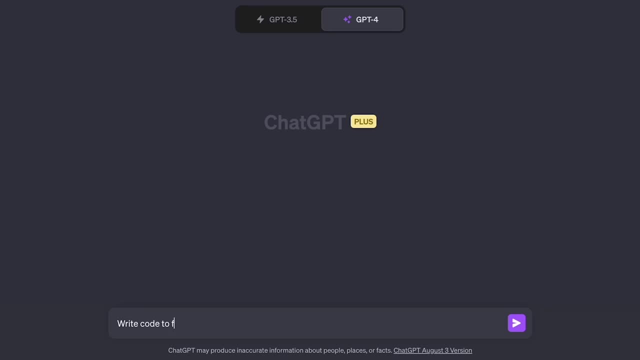 So in other words tokens that we are using, So in other words money- in order to get the right answer the first time. Here are some other examples of how you could write clearer prompts. So, for example, we have this prompt here which says: write code to filter out the ages from data. 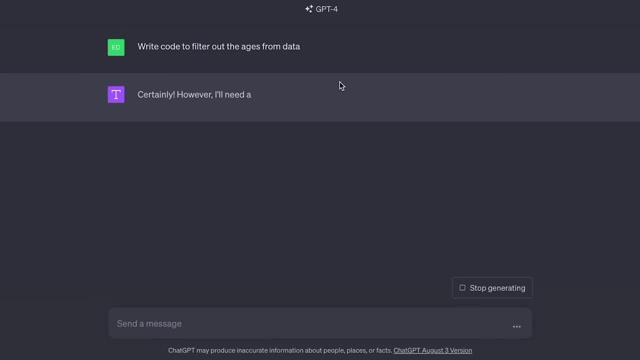 And if you run it, you don't really know what language is going to come back with. And if you run it, you don't really know what language is going to come back with. So, for example, here is using Python. I actually didn't want to use Python. 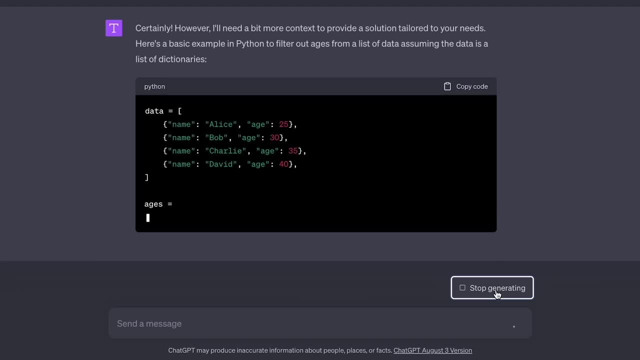 OK. so now we've lost some tokens asking this, We've also lost some time and we just haven't got the right response. This could have been so easily avoided. So I'm going to stop this from generating and let's try again. 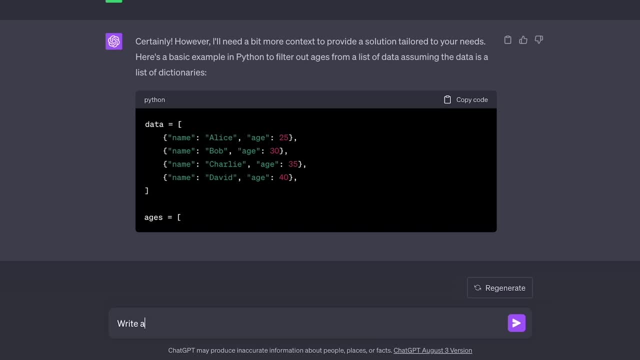 So this time let's be more specific by writing. write a JavaScript function that will take an array of objects and filter out the value of Age property and put them in a new array. Please explain what each code snippet does. In this example, I am not assuming the AI knows what computer language I like to use, and I am being more specific about what my data actually looks like. 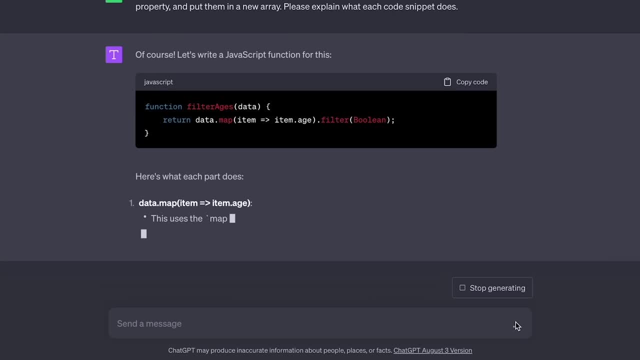 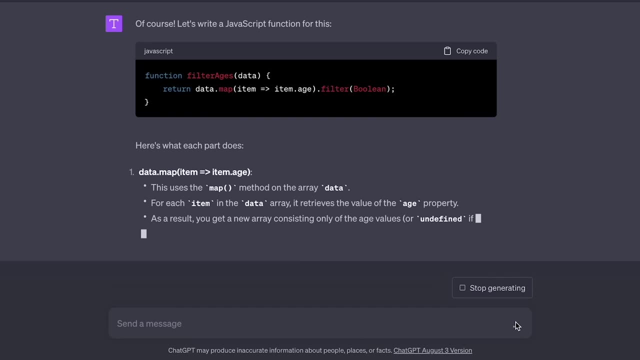 On this occasion, it's an array of objects. Not only that, I'm also asking the AI to explain why it's doing each step, so that I, in turn, can understand and not just copy paste the code without gaining any knowledge from it. OK, 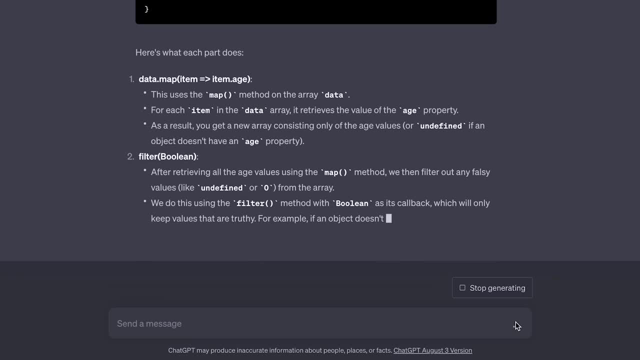 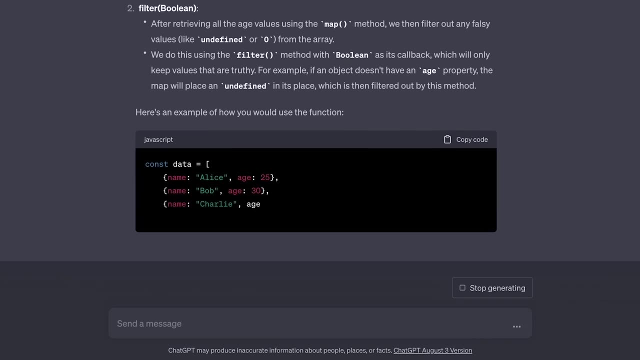 So here you can see a live example of what's coming back to us from GPT-4.. It's given us the correct code, So I have checked that and I was also giving us an example of how you would use the function, which is something I didn't ask, but it's super useful. 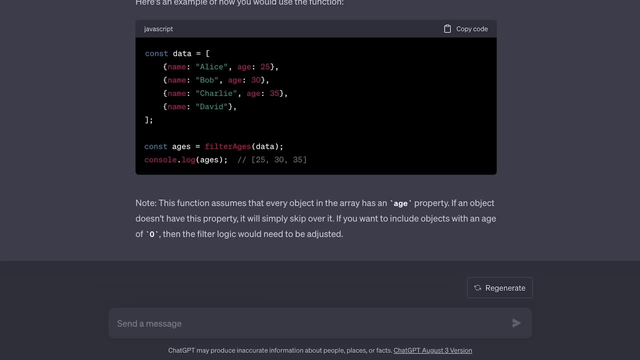 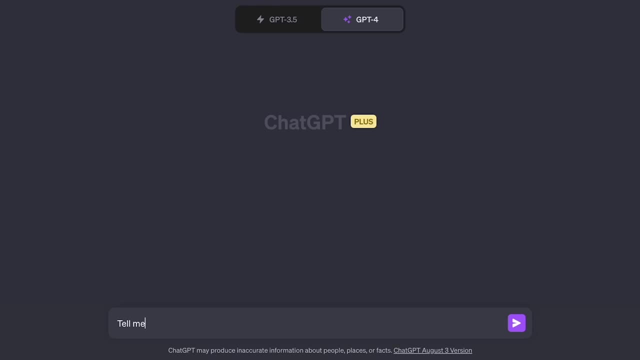 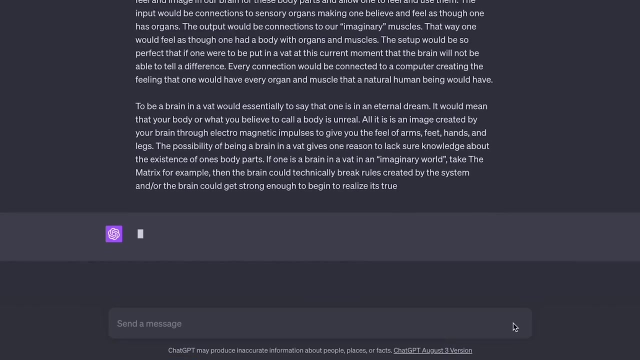 It's kind of gone above and beyond. for helping me out in understanding what is going on, Let's look at another example. We can write tell me what this essay is about. So I'm going to just type this and then just paste in an essay and hit go, and then ChatGPT will do its thing. 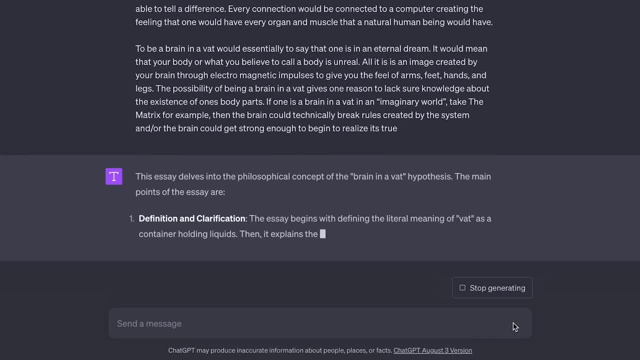 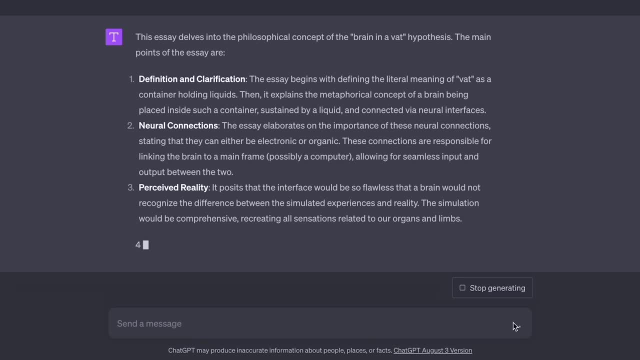 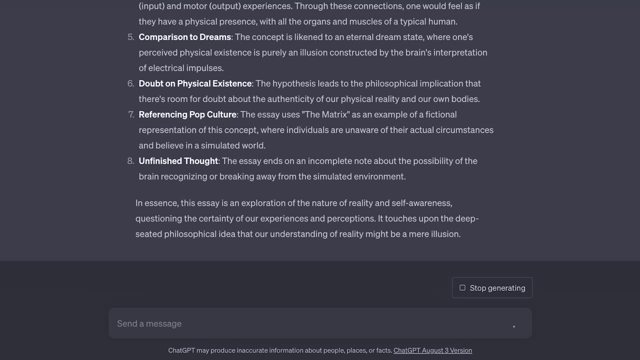 It's going to give me a summarization as it thinks best, So on this occasion it is essentially giving me numbered points about what this essay is about. They're really long. I really didn't want to read this much. It's pretty much looking to be the same as the original essay. 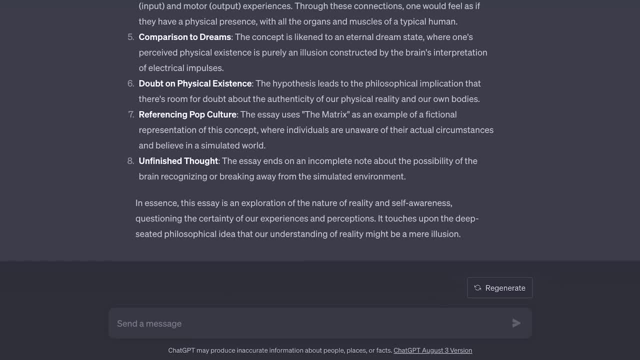 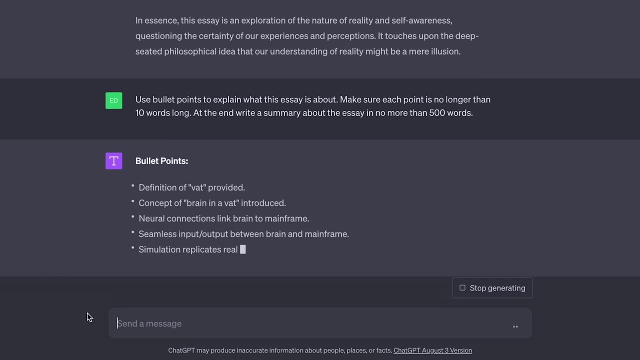 So this is not something I wanted. I should have been way more specific in telling it what I need. So what I'm going to do is just add to this conversation. So it's going to learn on what I wrote previously And I'm just going to specify, to use bullet points to explain what this essay is about: making sure each point is no longer the 10 words long. 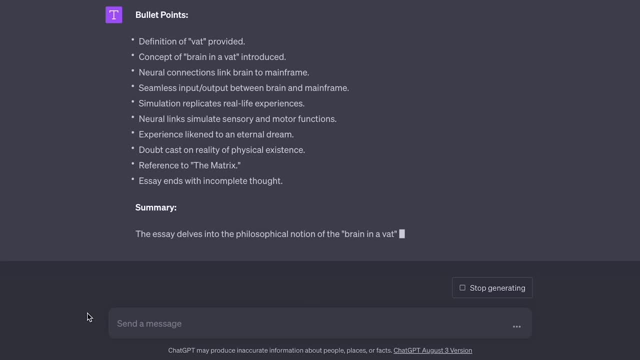 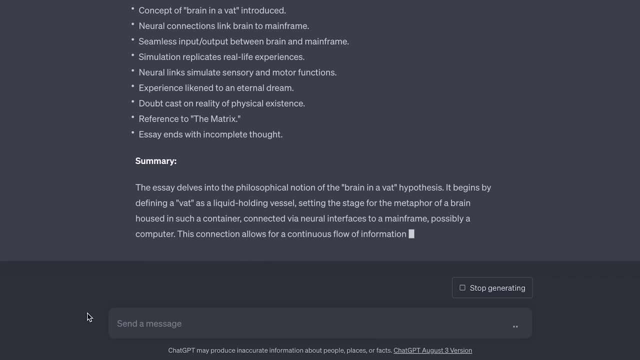 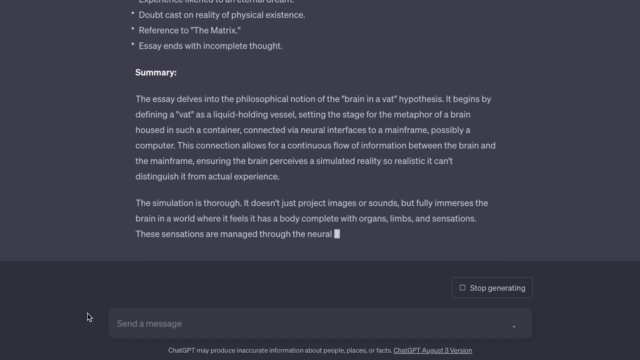 So I am being super specific in providing the instructions of what I want And let's hit go. So now this is a lot shorter. OK, as you can see, each point is no longer than 10 words long, And then I'm going to get a summary that is a bit longer and will give me a summary of the essay that I pasted in above. 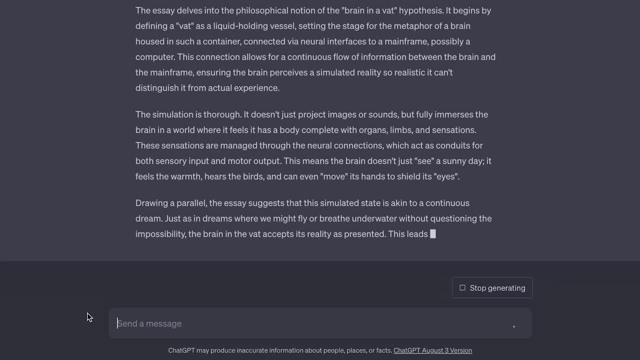 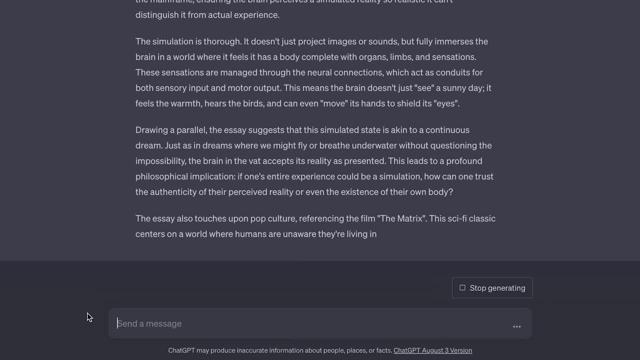 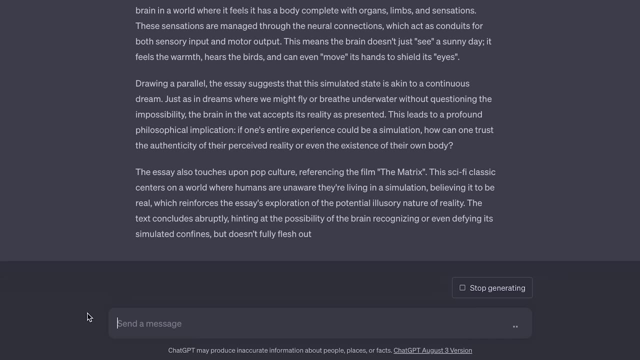 So great. Of course, you can do this on any essay or piece of text that you wish, and you can set your own clear and specific instructions as well. OK, so I hope you can see why the second one is better. It's because I am not assuming the AI knows what kind of format I want the summarization of the essay to be in. 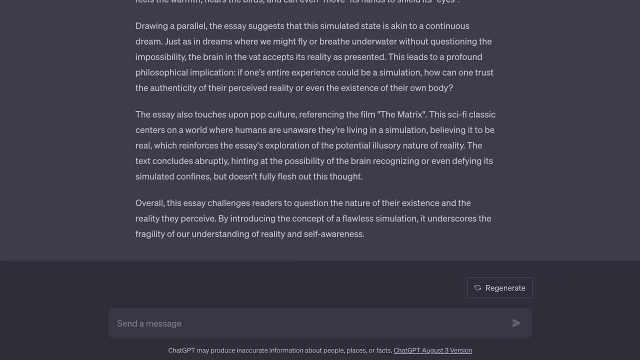 I am being specific, that I want very short notes on the essay in bullet point format, with a short conclusion at the end. If I did not put this, the summary could have been just as long as the essay itself, and the prompt could be considered useless in my eyes. 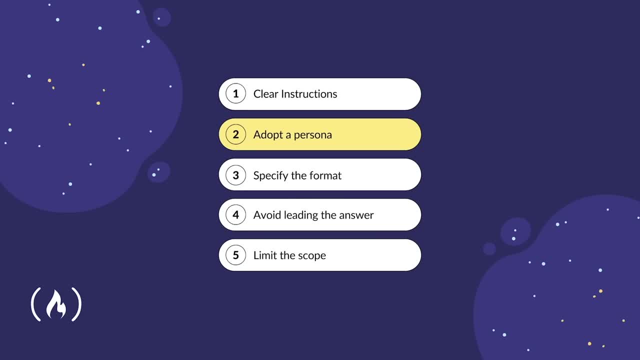 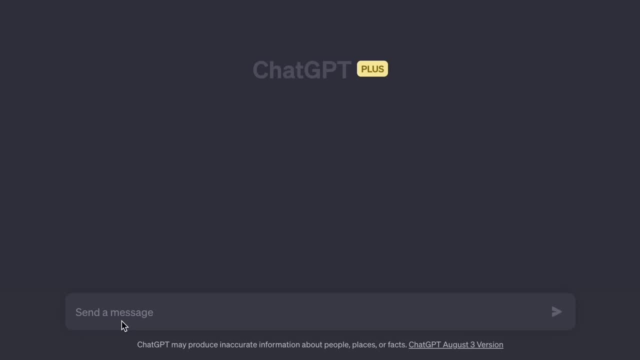 Next up, we can also adopt a persona. when writing prompts, It is sometimes helpful to create a persona. This means you are asking the AI to respond to you in a certain character. So, exactly like the English language teacher example we saw earlier, using a persona in prompt engineering can help ensure that the language model's output is relevant, useful and consistent with the needs and preferences of the target audience, making it a powerful tool for developing effective language models that meet the needs of users. 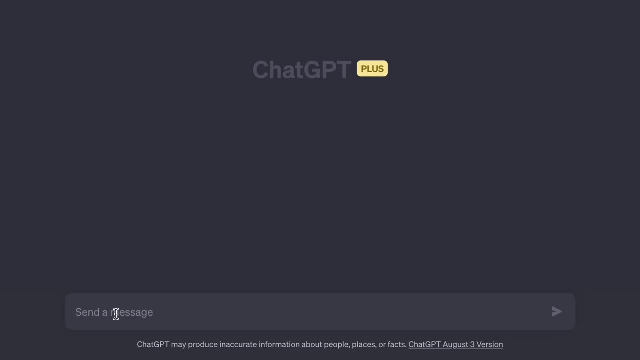 Let's look at some examples of adopting a persona. So, for example, you can have This prompt right here: write a poem for a sister's high school graduation that would be read out to a family and close friends. So let's go ahead and run this and let's see what comes back. 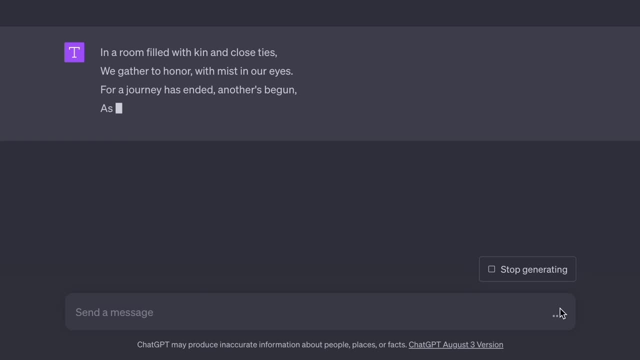 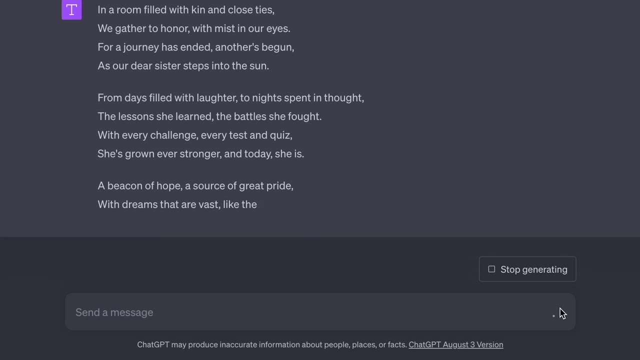 So there we go. It is quite good. in a room full of kin and close ties, We gather to honor the mist in our eyes, for a journey has ended, Another begun as our dear sister steps into the sun. OK, so it's coming out with a poem I can see here: 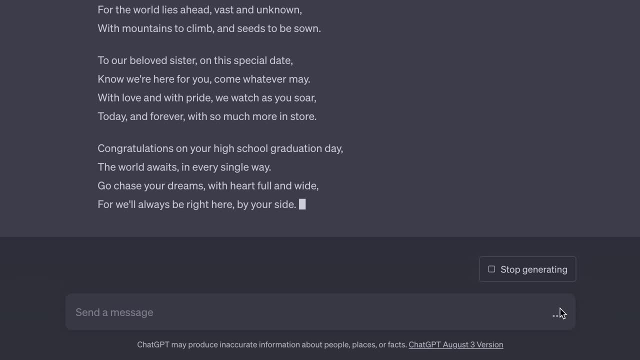 It is quite a good one, I guess, probably better than anything that I would have written, And it is maybe a little bit generic. Maybe that's what you wanted. I think we can do better than this, So let's try this. 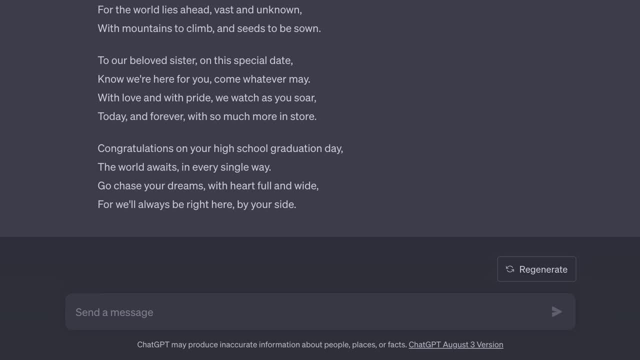 This time I'm going to write a prompt with a persona, So this time I'm going to specify who I'm writing as I'm going to do: write a poem as Helena. Helena is Twenty five years old and an amazing writer. Her writing style is similar to famous 21st century poet Rupi Kaur. 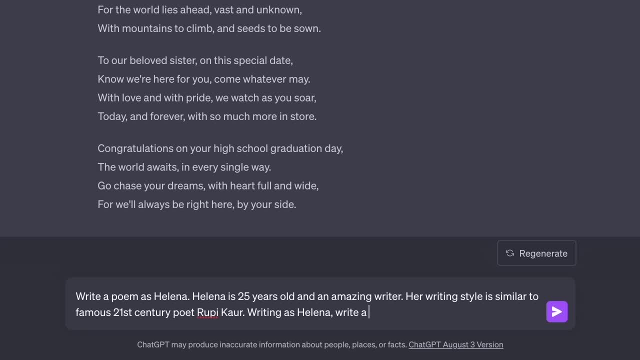 Writing. as Helena write a poem for her 18 year old, I'm going to write a poem for her sister to celebrate her sister's high school graduation. This will be read out to friends and family at the gathering. OK, so let's check it out now. 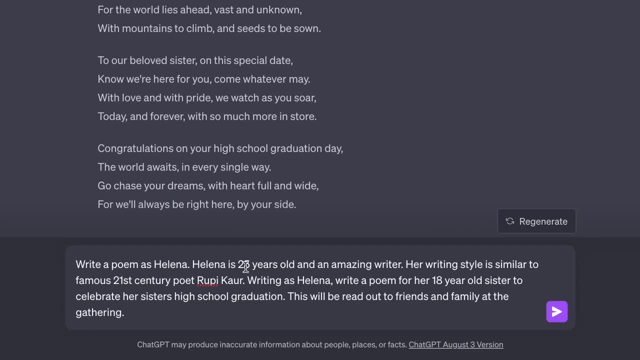 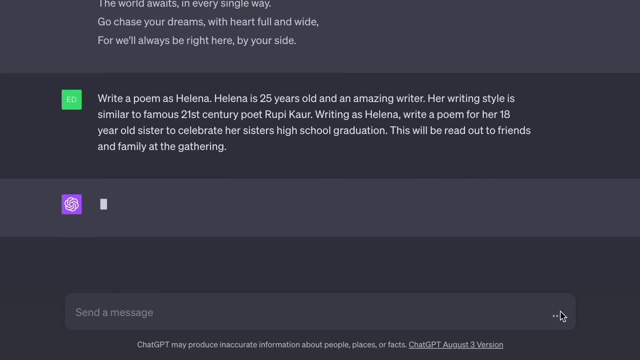 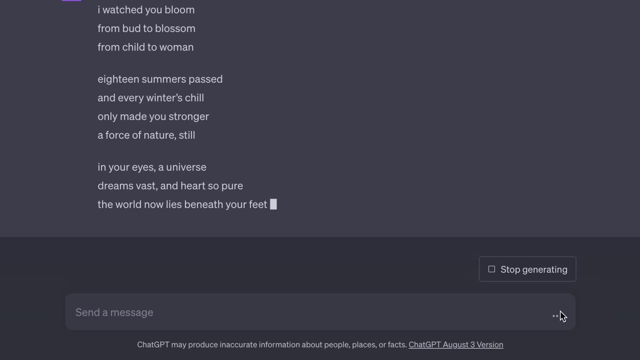 We're writing as Helena, She's 25.. She's an amazing writer And we've also assigned a writing style, So let's check it out now. Chat GPT should be using anything it knows about Rupi Kaur, hopefully from the Internet, in order to apply that style to this poem. 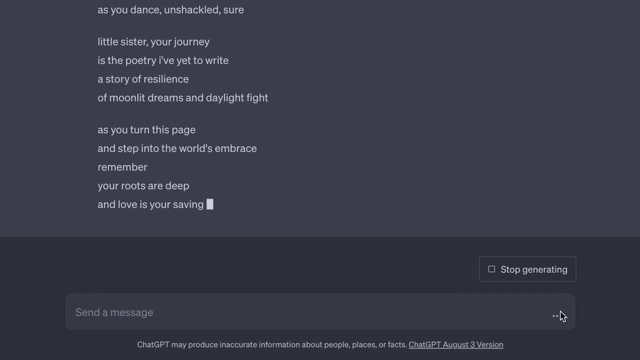 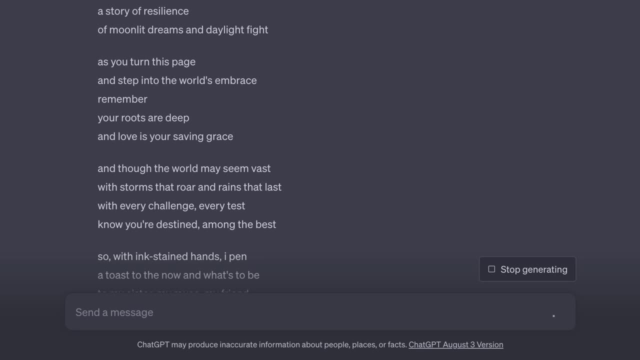 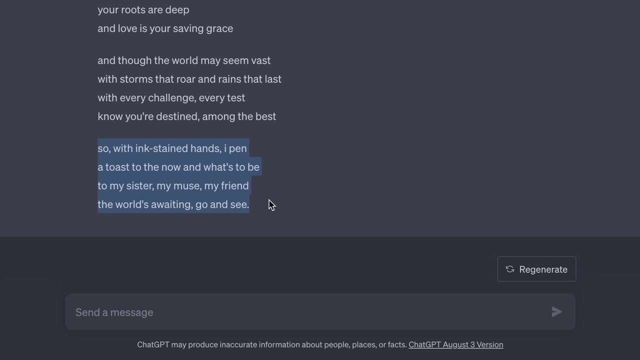 OK And, as you can see, this is maybe a little bit more affectionate. We've said sister. It's obviously a younger sister, So the words little sister are being used And, in general, OK, general. I think this is a much higher quality poem and if Helena truly does have the style of 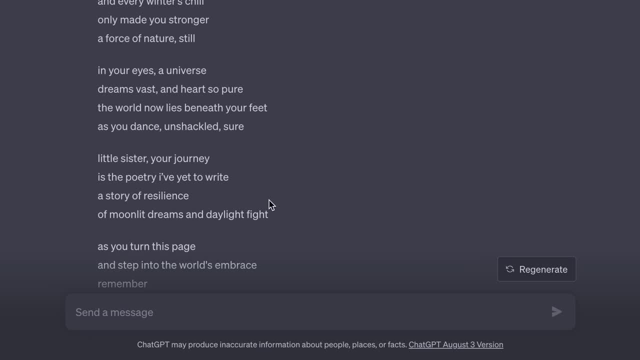 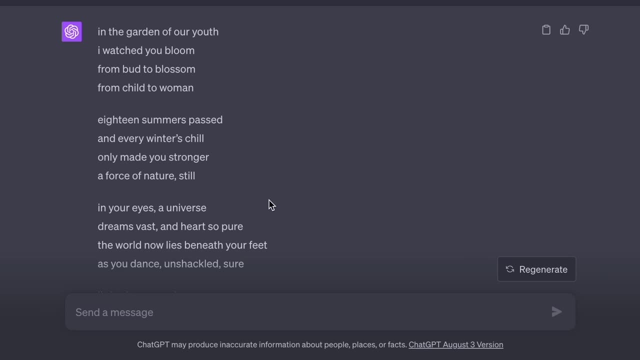 Rupi Kaur. in writing. it will be almost indistinguishable who wrote this poem: chat GPT or Helena. So here we go. here's the full thing. it starts off in the garden of our youth. I watch you bloom from bud to blossom, from child to woman, 18 summers past. again utilizing the fact, 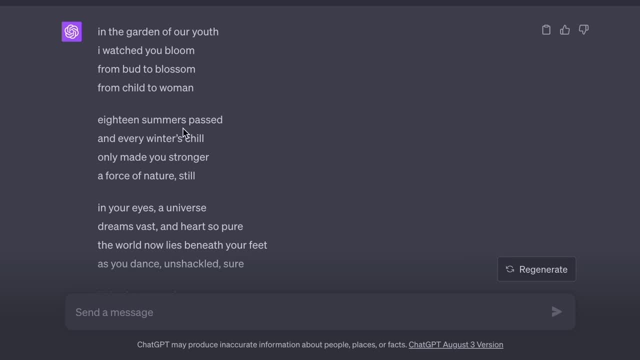 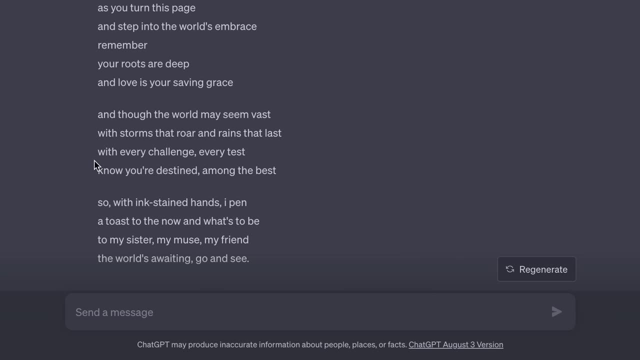 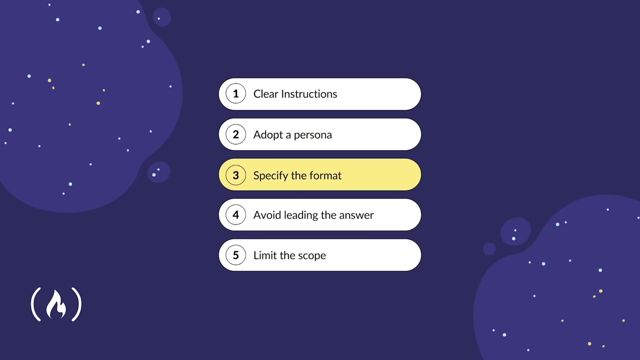 that we fed it. she was 18, and every winter's chill only made you stronger- a force of nature still so, yes, in my eyes, this poem is a lot more better. it's much more refined, it's much more personal, thanks to the prompts that we wrote. We've already had a brief look at specifying format. 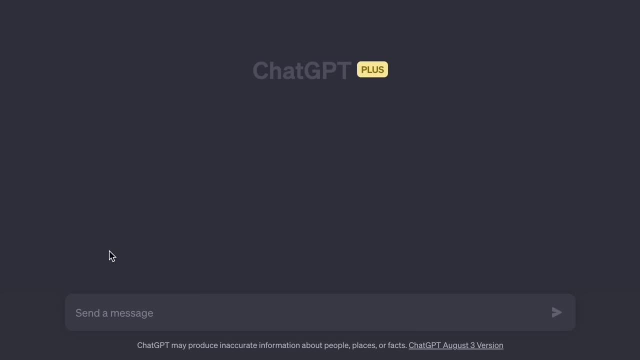 when we limited the word count of our bullet points in a previous example. so that was a great example. limiting words is one that I use often. however, we can do a bunch of other things, including specifying if something is a summary, a list or a detailed explanation. Heck, you can even create checklists, so I'm going to go ahead and show you. 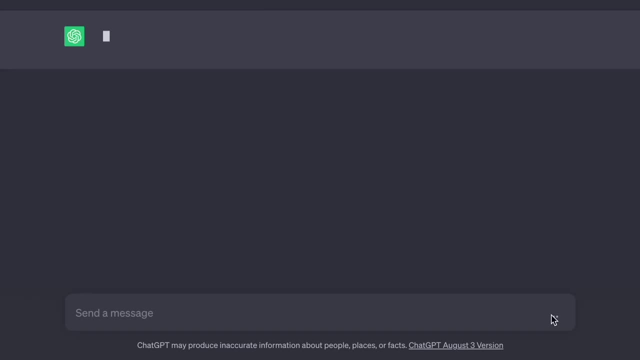 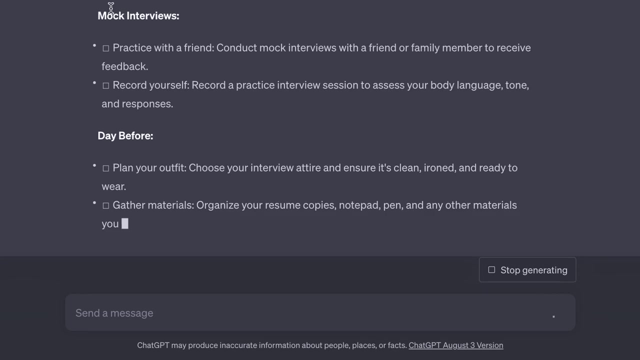 how to do this. here is an example prompt and I'm just going to run it. and there we go. we have created a checklist. so many things you can do in chat, GPT. just make sure to specify the type of a word you want to use, and if you do that, you will get a lot more information about the. 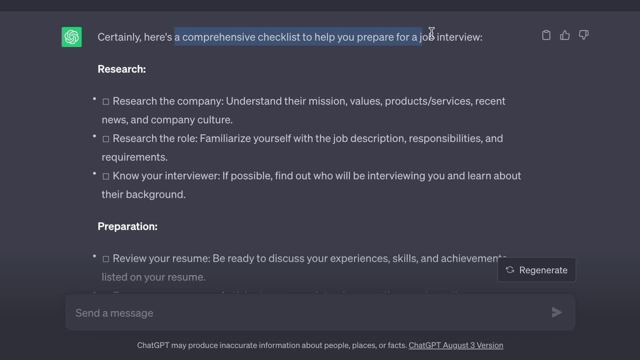 format you want, and it should be able to do it. Okay, great, now that we looked at some best practices, let's move on to some more advanced topics. in the prompt engineering In this section, I'm going to talk about two types of prompting. we can. 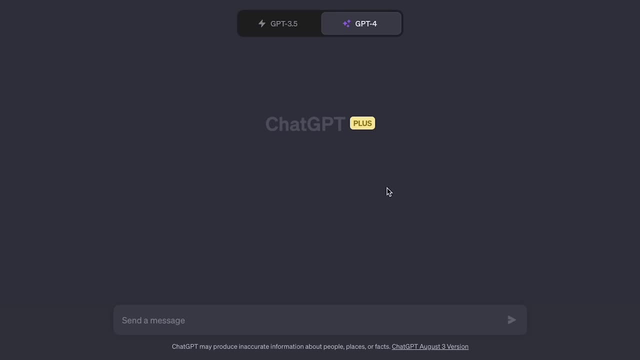 do Zero-shot prompting and few-shot prompting? Zero-shot prompting leverages a pre-trained model's understanding of words and concept relationships without further training, and few-shot prompting enhances the model with training examples via the prompt, avoiding retraining. So essentially in the context, 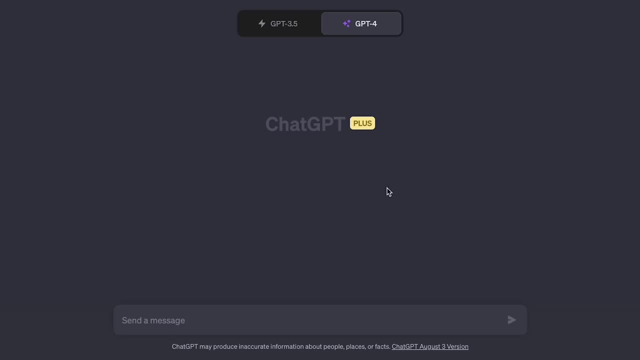 of the GPT-4 model. we don't really need to do much. we are already using all of the data that it has in order to ask when is Christmas in America. So let's go ahead and do some zero-shot prompting- when is Christmas in America- and hit. 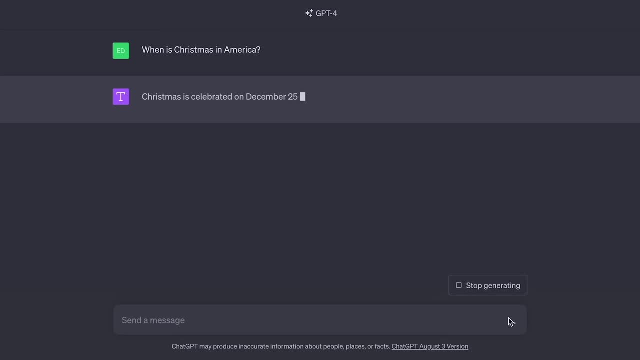 zero Go. Okay, so it clearly already has the data for this. we don't need to add any examples or anything like that. So, as you can see, zero-shot prompting refers to a way of querying models like GPT, without any explicit training examples for the. 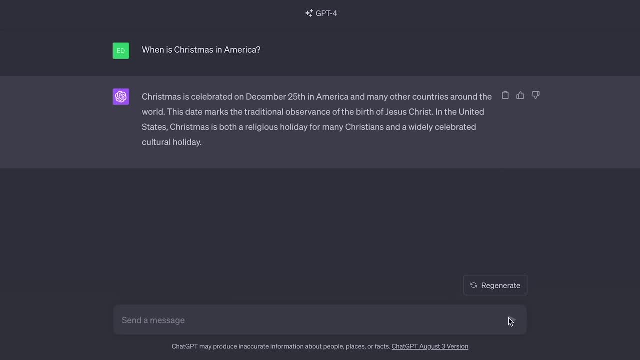 task at hand In the context of machine learning, and not just GPT. zero-shot typically means that a model performs a task without having seen any training examples for the task at hand In the context of machine learning, and not just GPT. zero-shot typically means that a model performs a task without having seen any 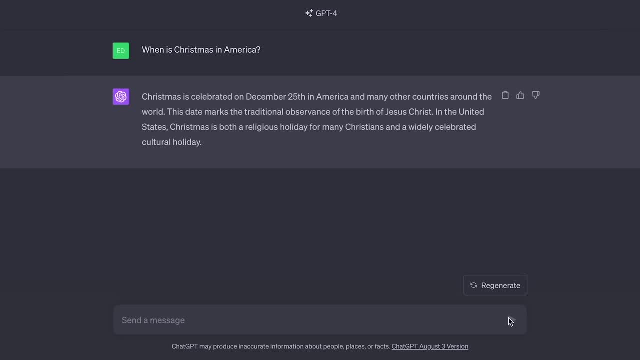 examples of that task during its training. Okay, great. so now let's look at few-shot prompting. So once again, with zero-shot prompting, we give our language model a prompt and got a response, but sometimes that's just not enough and we need a bit more training. so let's use few-shot prompting and level up our 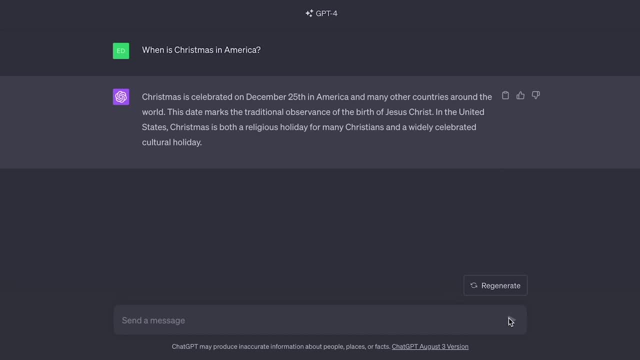 language model by showing a few examples of the task we want it to perform. So instead of zero example- we give it a tiny bit of data. So let's think: what would GPT-4 not know? I guess it would not know my favorite types of food. So, for example, let's check what is Ania's favorite type of food. 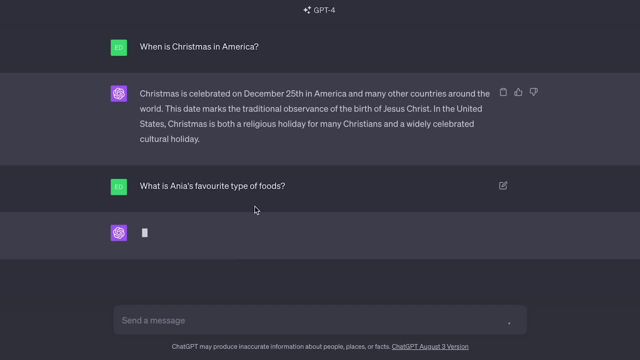 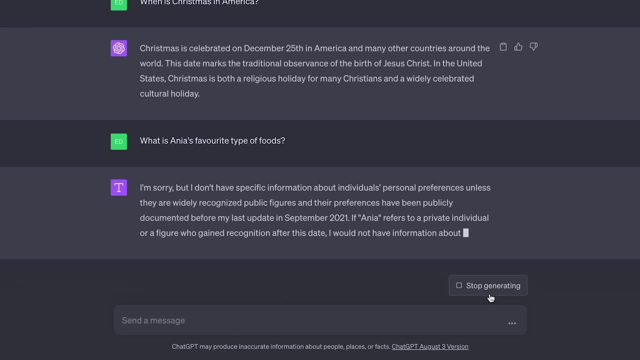 Plural Okay, And I mean it can guess, but no, it's just telling me that it doesn't know. So that is absolutely fine, Let's stop generating. So now, let's feed it in some example data. I'm 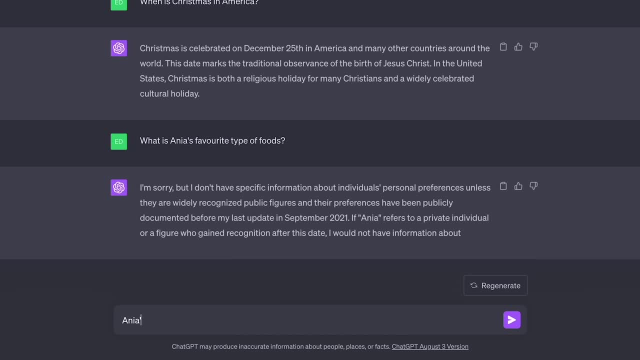 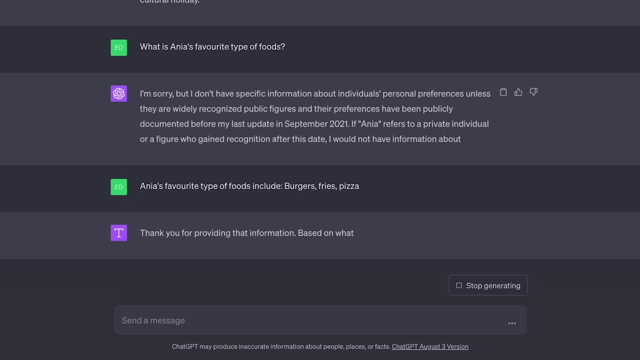 going to feed it in a tiny bit of data. Ania's favorite type of food include: sorry about my English, Let's go with burgers fries- I love fries pizza. and hit enter. Okay, So we are essentially giving chat GPT some information. Uh, so now if I type, 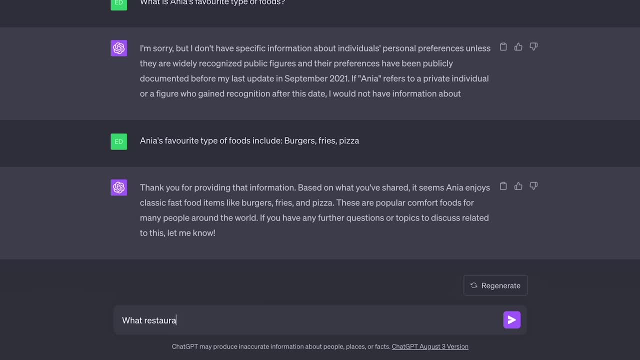 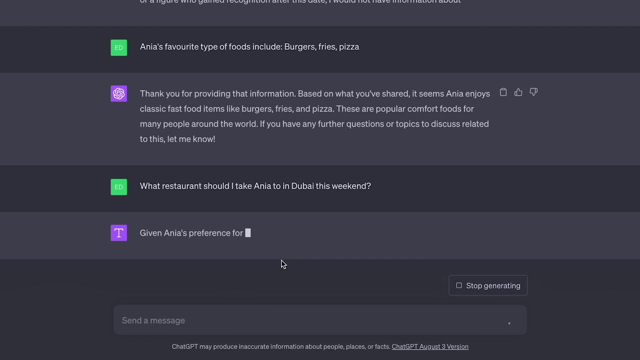 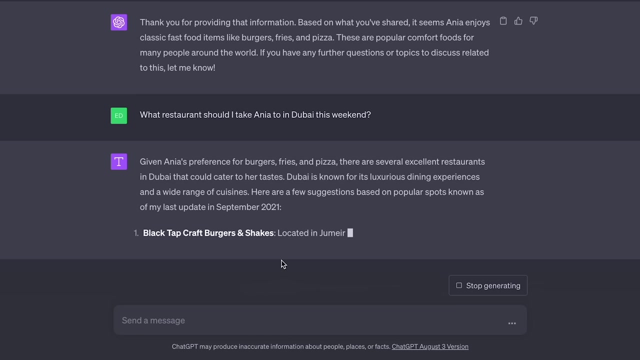 what restaurant should I take Ania to in Dubai this weekend and hit here? it should hopefully understand that my favorite types of foods are burgers, fries and pizza And, given that, find me some restaurants in Dubai that I would like to go to, So here are some. this has been. 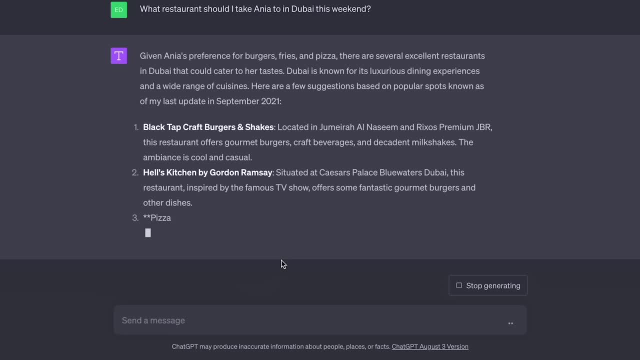 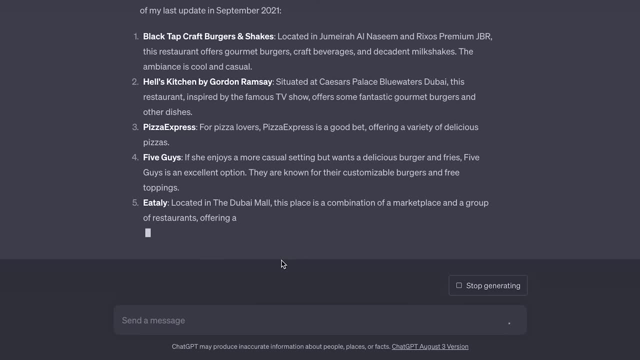 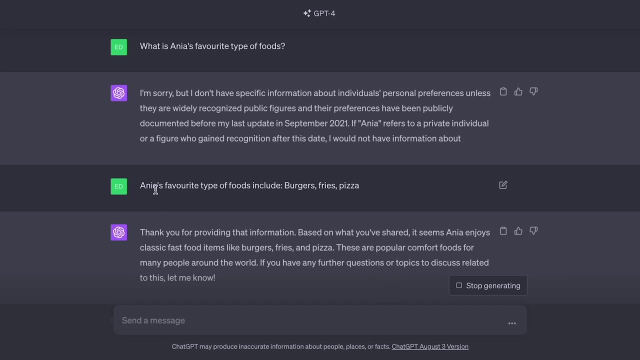 updated as of September 2021, but you know these are pretty good ones, So I would totally go to these. This is a great example of few shop prompting in which it wouldn't have been able to answer this question if I hadn't had given it some example data or just trained the model a little. 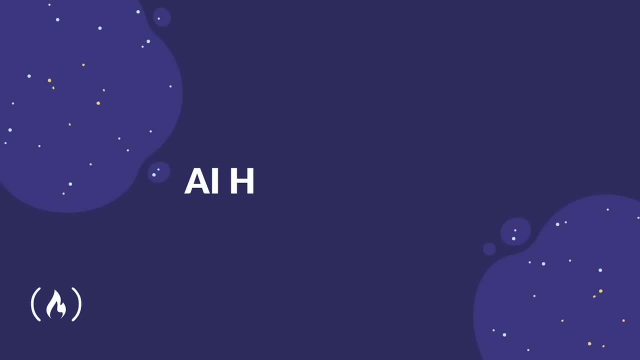 bit more, But this is a very, very good example of where you can actually get some help with your AI. Okay, So here are some of the questions that were asked in this video. The first one is this question that I have been given multiple times: 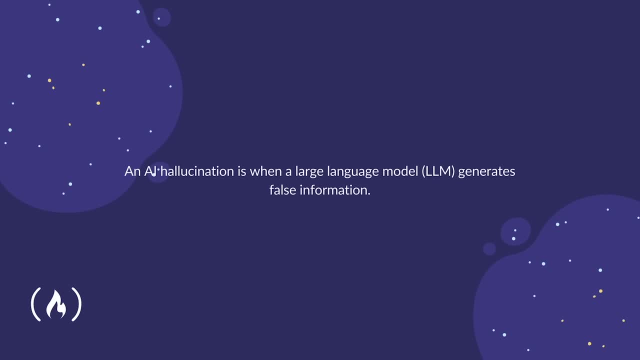 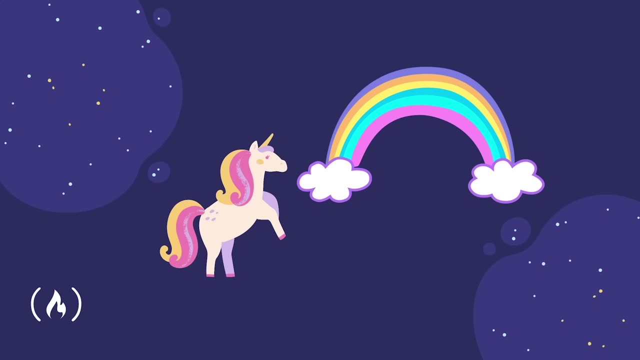 this is a really interesting question. I've been trying to figure out what my AI models and what my AI models can do to improve my AI performance in an AI context. It's actually a really good question. It's actually a really nice to hear some of the 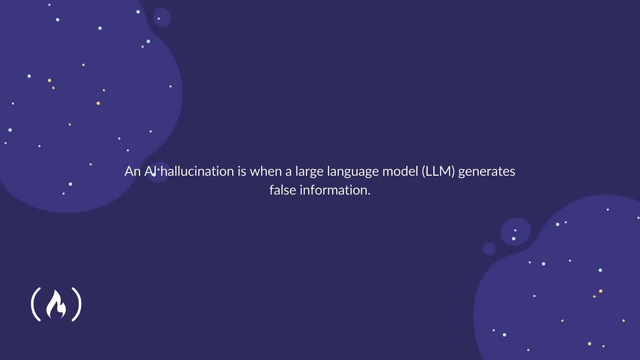 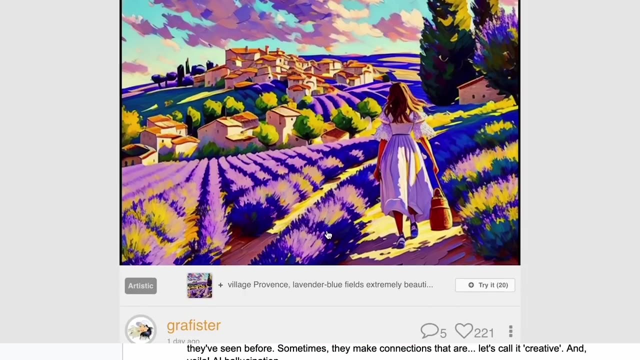 answers to- and it is great- data. Now I think I'll give you the answer here. I think you may be able to understand this question better than the rest of the example of this is Google's deep dream. you know, that project that turns. 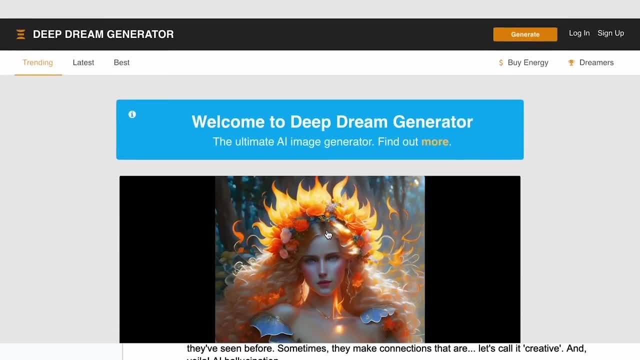 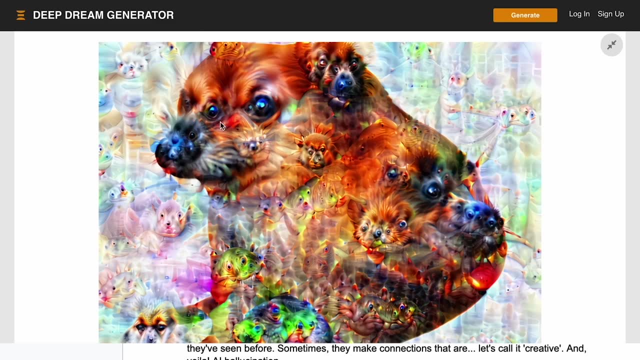 pictures of your dog into a nightmarish blend of dog faces and well more dog faces. deep dream is an experiment that visualizes the patterns learned by a neural network. it is built to over, interpret and enhance the patterns it sees in an image, or in other words, fill in the gaps with images. but some of the 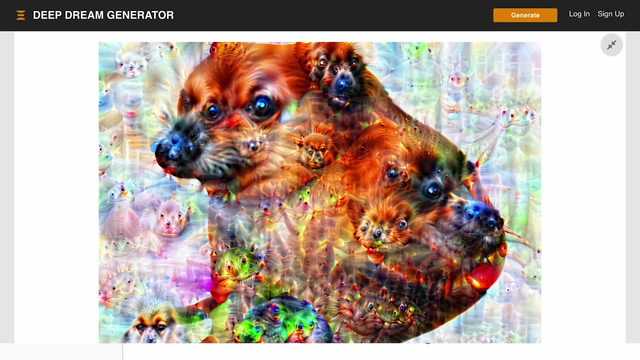 time, those gaps can be filled with the wrong thing. this is an example of an unusual output the AI models can produce when they miss interpret data. now, why do these hallucinations happen, you ask? they're trained on a huge amount of data and they make sense of new data based on what they've seen before. sometimes, 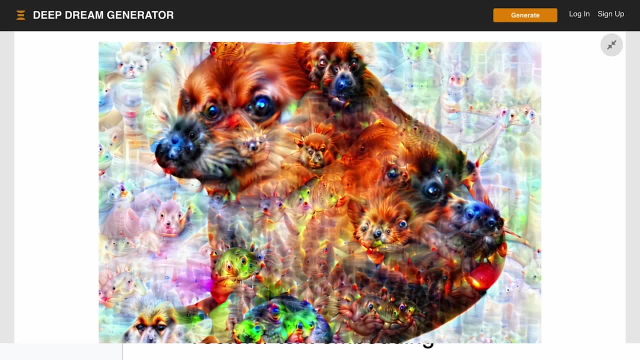 however, they make connections that are- let's call it- creative and voila, an AI hallucination occurs. despite their funny results, AI hallucinations aren't just entertaining, they're also quite enlightening. they show us how our AI models interpret and understand data. it's like a sneak peek into their 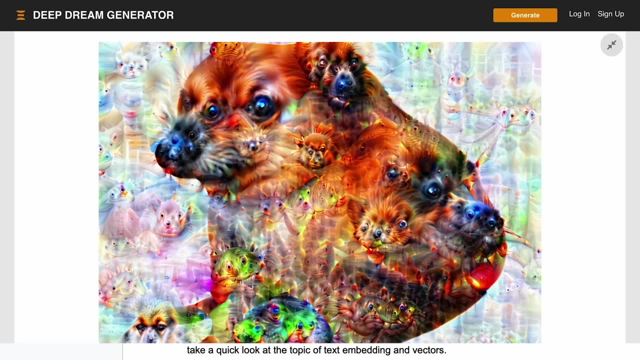 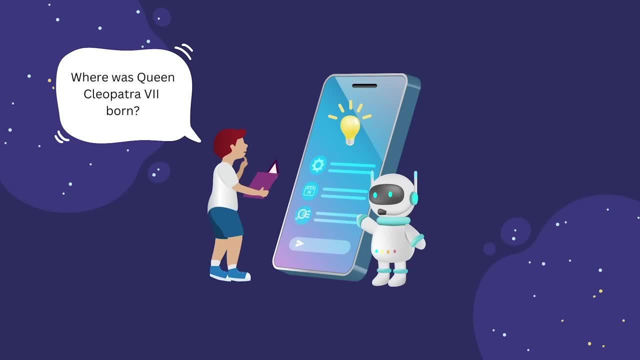 thought processes. this example is actually an AI image hallucination, as I thought it would be a fun one to show. AI hallucinations can also happen with text models. an example of this is us asking a text model about a historical figure and the text model not having an answer, and 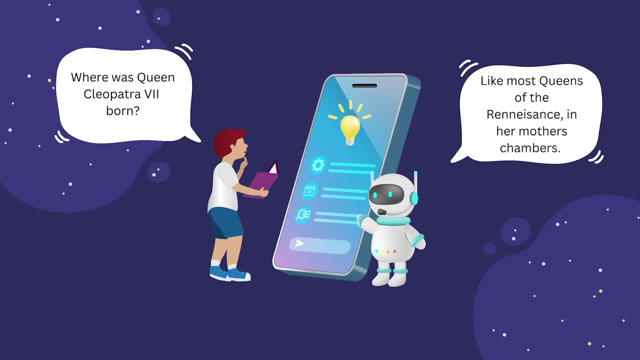 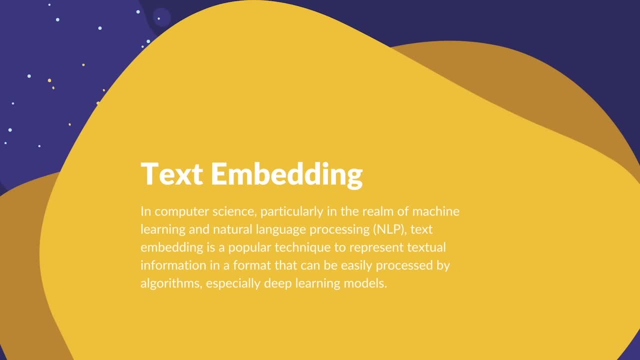 hallucinating one, instead resulting in an inaccurate response. vectors and text embeddings. to finish off, I'm gonna leave you with a slightly more complex subject. we are going to take a quick look at the topic of text embedding and vectors in computer science, particularly in the realm of machine learning and natural 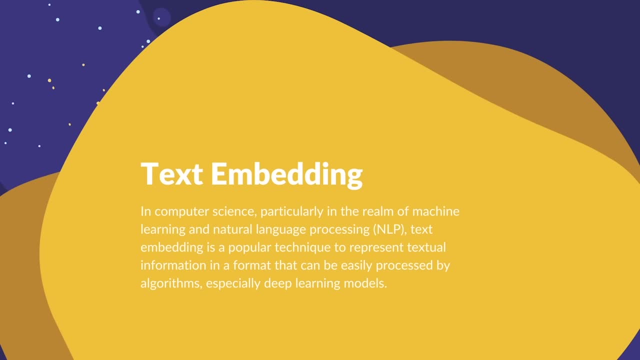 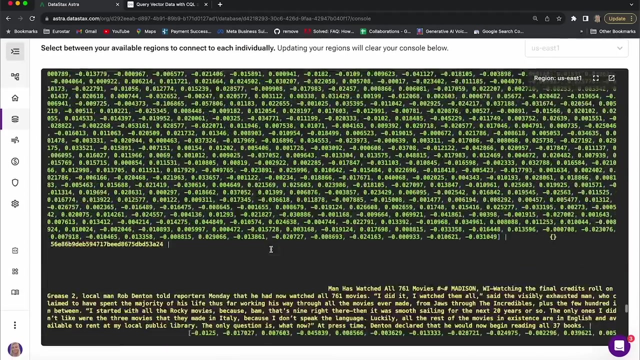 language processing or NLP tax. embedding is a popular technique to represent textual information in a format that can be easily processed by algorithms and especially deep learning models. In the context of prompt engineering, LLM embedding refers to representing prompts in a form that the model can understand and process. This involves converting. 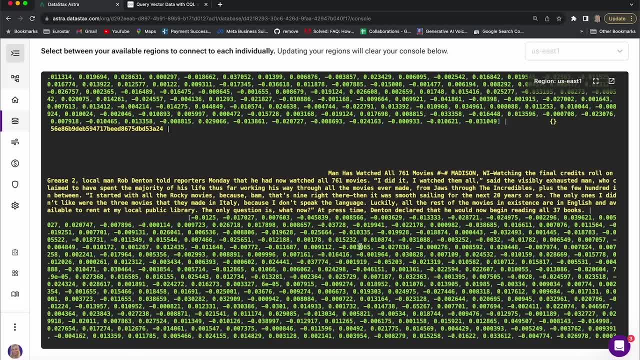 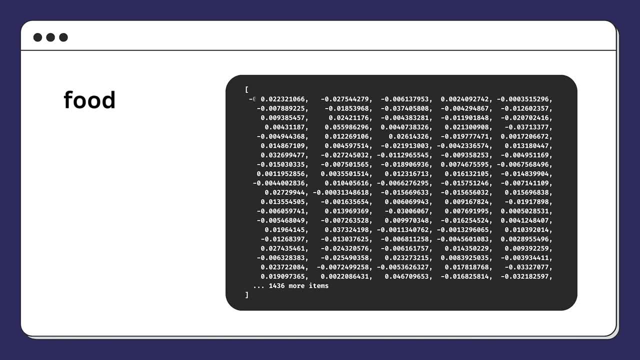 the text prompt into a high dimensional vector that captures its semantic information. So, essentially, the word food is represented by this if using the create embedding API from open AI. Okay, so you will see it represented. the word was represented by an array of lots and lots of. 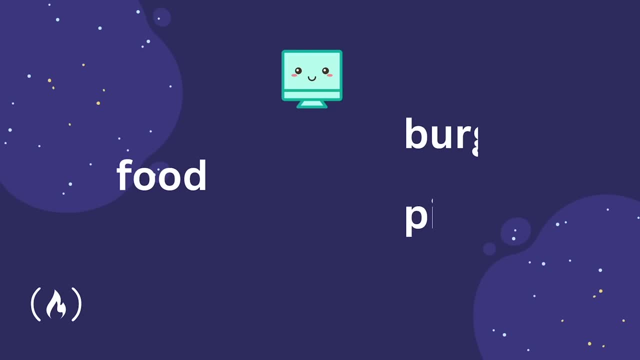 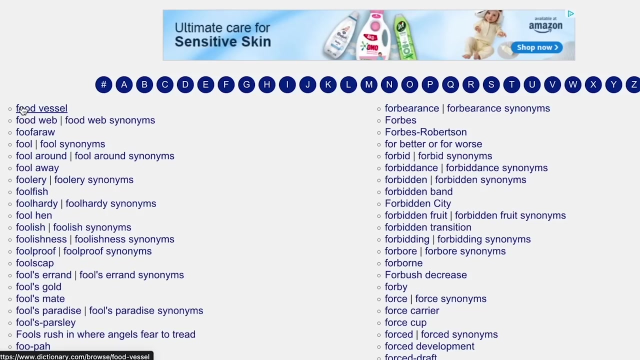 numbers. But why do this? Well, think about it this way: If you ask a computer to come back with a similar word to food, you wouldn't really expect it to come back with burger or pizza, right? That's what a human might do when thinking of similar words to food. A computer would more. 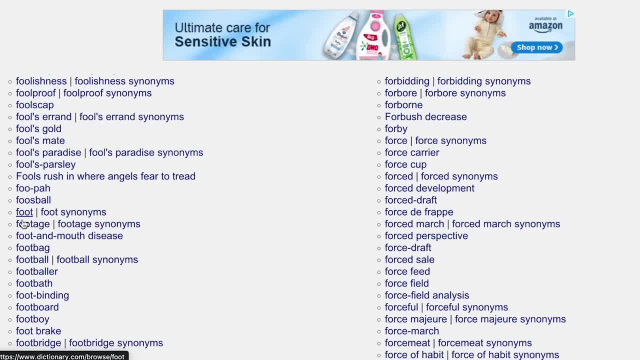 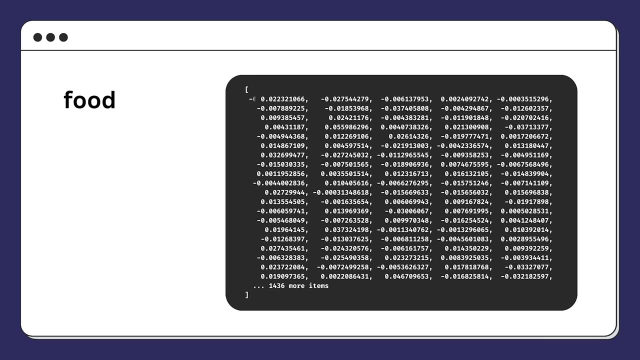 likely look at the word lexicographically, Kind of like when you scroll through a dictionary dictionary and come back with foot, for example. This is kind of useless to us. We want to capture a word's semantic meaning, so the meaning behind the word. Text embeddings do. 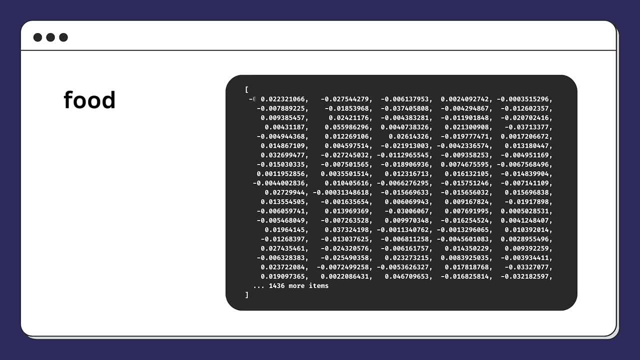 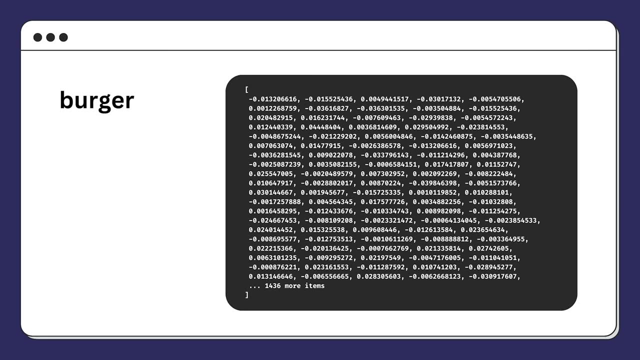 essentially that, thanks to the data captured in this super long array, Now I can find words that are similar to food in a large corpus of text by comparing text embedding to text embedding and returning the most similar ones. So words such as burger instead of foot. 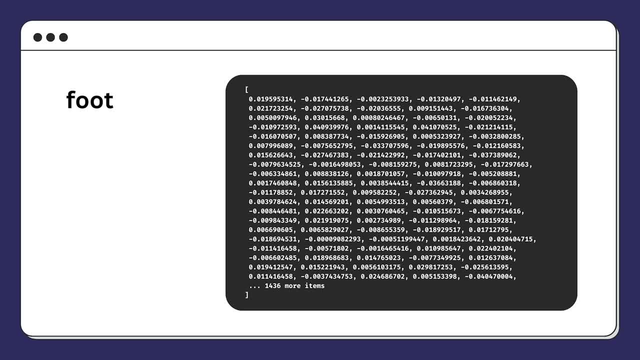 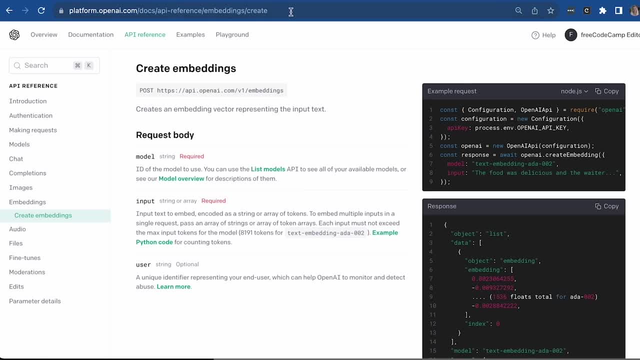 will be more similar To create a text embedding of a word or even a whole sentence. check out the create embedding API here from OpenAI. So here's the URL that you should visit And to create your own text embedding, you're going to have to create a post request to. 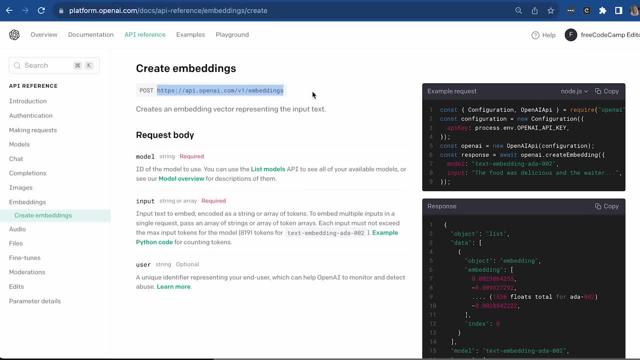 this endpoint. Okay, so that's what you can do. You can also take the code from here. So this is an example request written in Nodejs, And you would have to install the OpenAI package. take these two methods from it in order to. 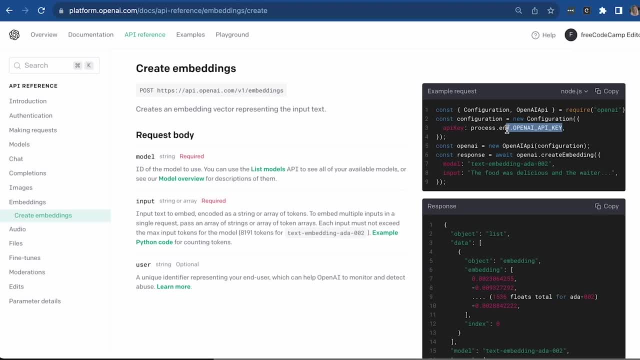 pass through your OpenAI API key. that I showed you how to get earlier. As a refresher, you should go here and view API keys to create your own API key And once you pass that through, you can then use the const configuration and pass it through here in order to use OpenAI.